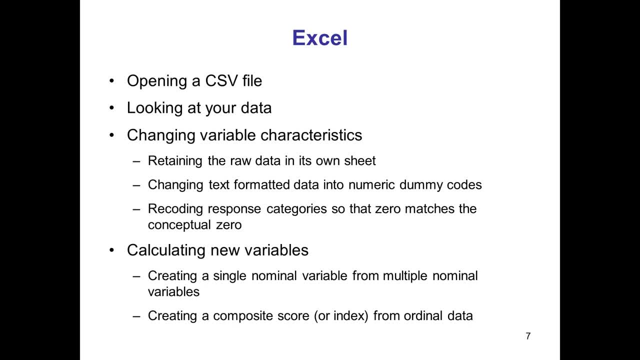 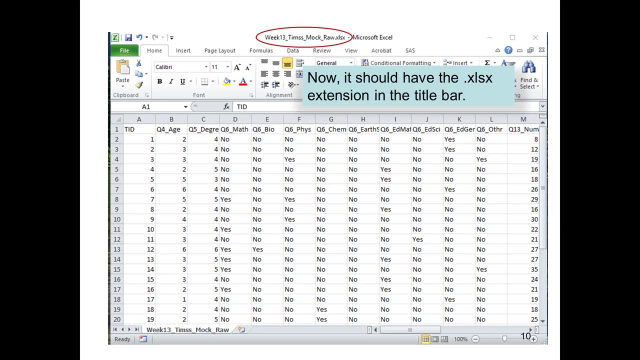 rules of Dilman, Smyth and Christian. You can go through all of the Excel files here And basically, when we go to the R code, which we'll do momentarily- and that R code goes in the same order as the slides in Excel. 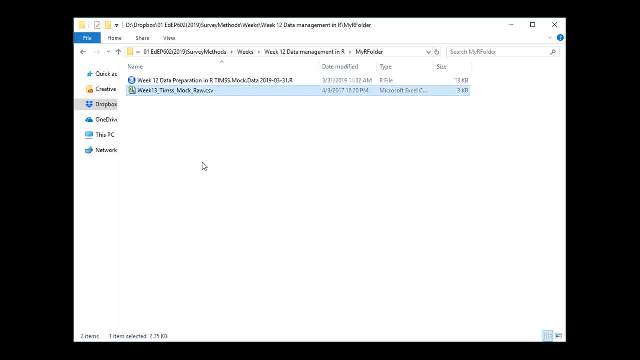 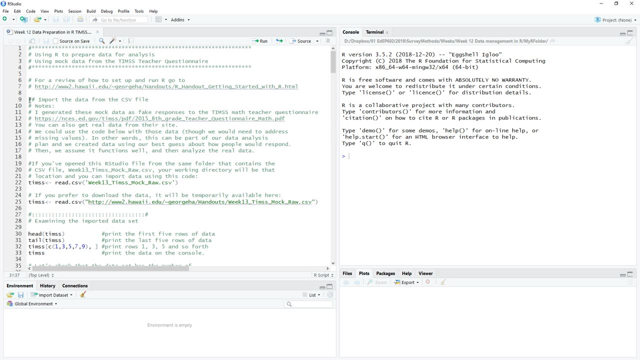 I have my R file and my data file in the same folder. This makes it easy for my working directory. I don't have to specify it when I switch computers. So you click on your R file and this is our R file. So basically I explain how you can import the data file. 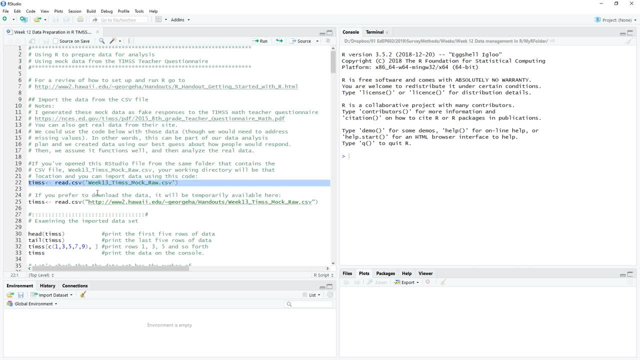 Now here's our line of code for importing it from the directory where I just was. If you prefer to download it from the web page, you can do it this way. So I just highlighted this and I click Run. Then I can examine my data. 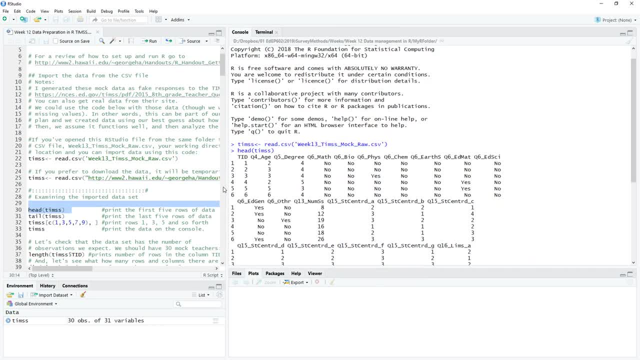 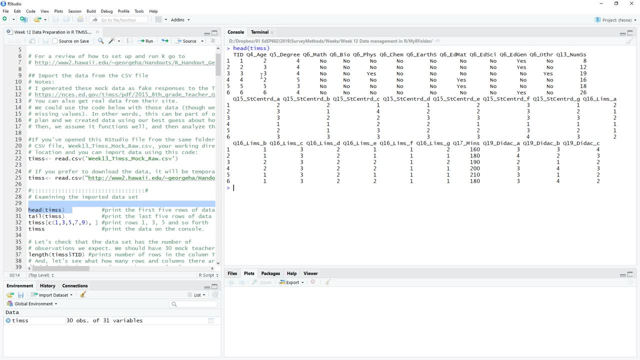 So I can see. oh okay, Let me clear my ID of Control-L or Command-L. I can examine my data and I can see I have teacher ID as a a variable or a column, the age, the degree of a person. 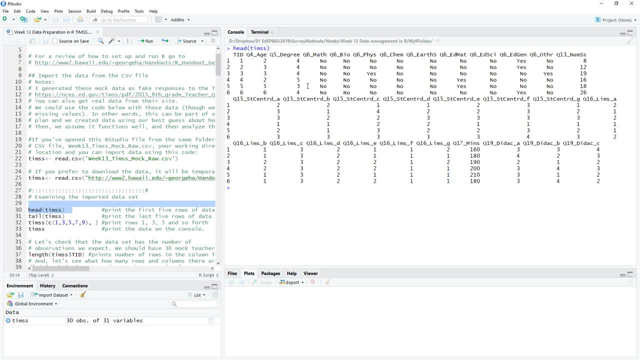 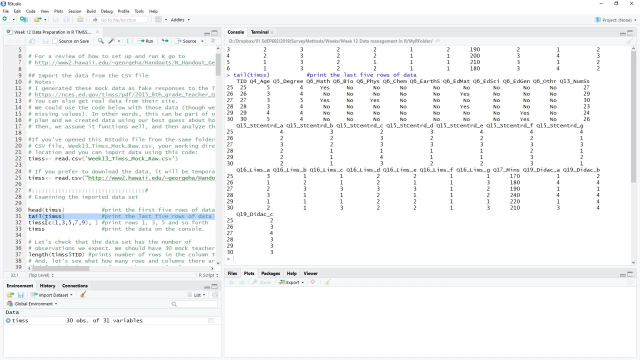 which is coded according to that PDF of the TIMS, whether they majored in mathematics or biology and so forth, And so those are demographic variables, And so we can examine our data. using the heads and the tails functions. We can also look at specific rows. 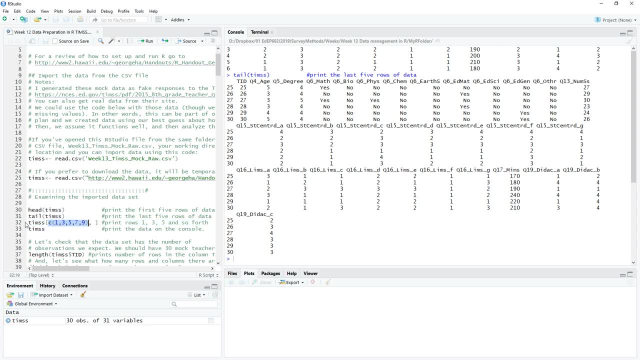 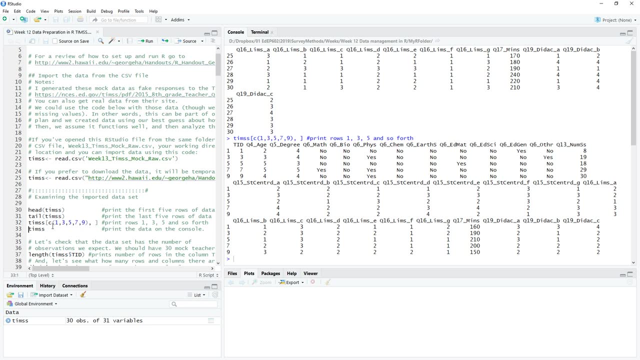 So this is before the column within the brackets. So I can look at rows 1,, 3,, 5,, 7, and 9, and it'll show me those ID responses. I could also just look at the entire data set. 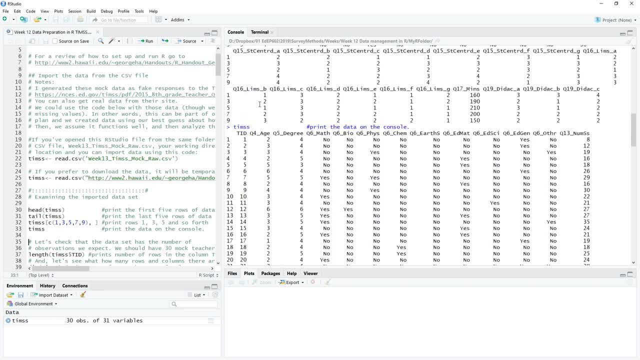 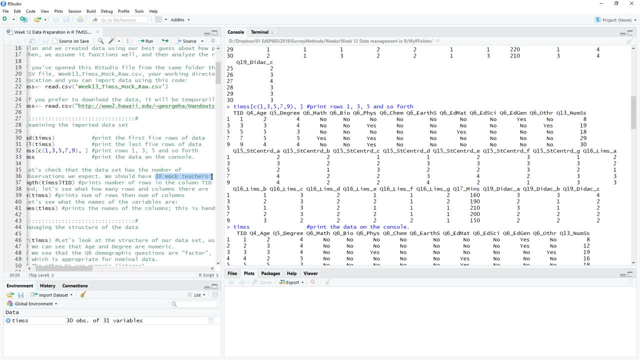 And if it's not too long it will all show up in the console here And I want to make sure that I have imported it correctly. I'm expecting to have 30 mock teacher responses So I can look at the length of my data set. 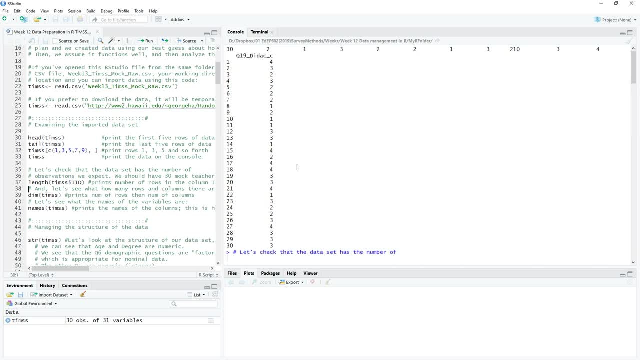 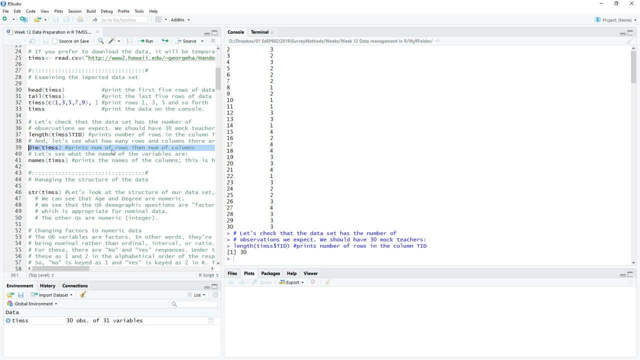 Maybe I'll look at the length of my teacher ID variable, and it should be 30. And the result is indeed 30.. Let's see, I could also use the DIMM function to see the same thing. This will give me how many rows and how many columns. 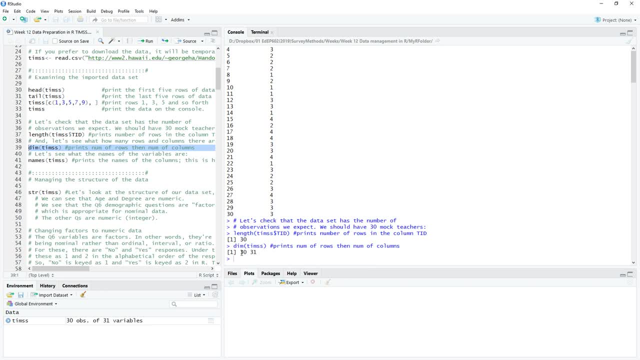 So there are 30 rows and 31 columns, So that means I have 31.. I guess you could call them variables. They're not necessarily variables, They're columns. I can see what are the names of those columns, because this is a data frame. 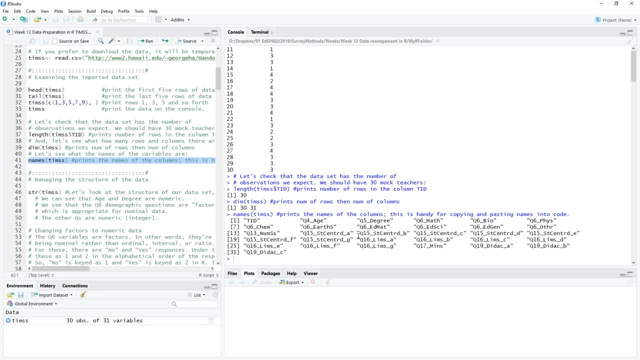 and so it lists what they are. So this is handy when you're running code and you want to go see. oh, what was the name in my data set of the first portion of question 15?? Yeah, so it's Q15 underscore. 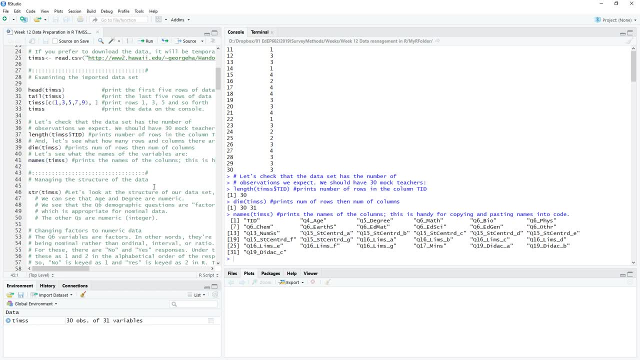 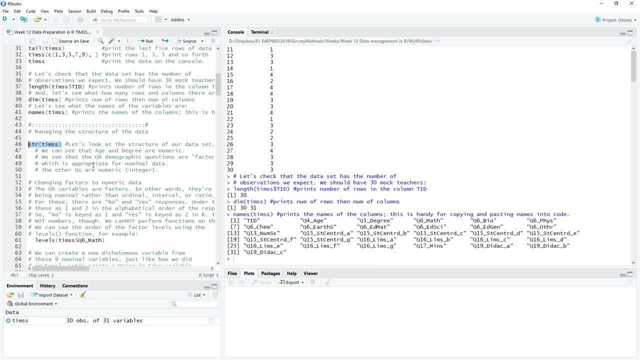 So I could actually copy that and then I could put it in my code somewhere. you know when I wanted to run it. So that's valuable. I want to see how the data are structured in R, So I use this STR function. 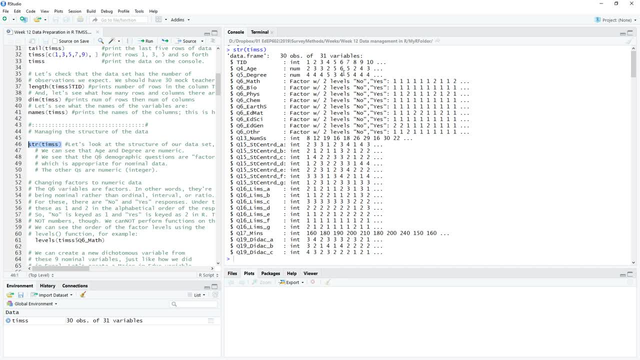 And this tells me that teacher ID is integer, which is interesting, probably because it just automatically RR. Yeah Yeah, It automatically detected it as numeric integer because there were no decimal places. But you know, if I had names, then teacher ID would be a character variable. 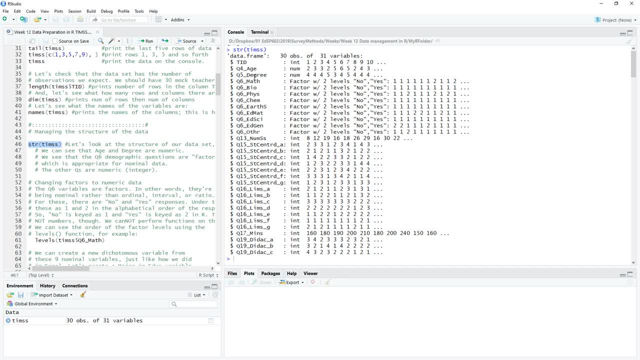 We don't have any character variables in here. Age and degree are numeric. I guess I think in the Excel file they had a decimal. In the CSV file there was a decimal place with two zeros after. So R interpreted that as numeric. 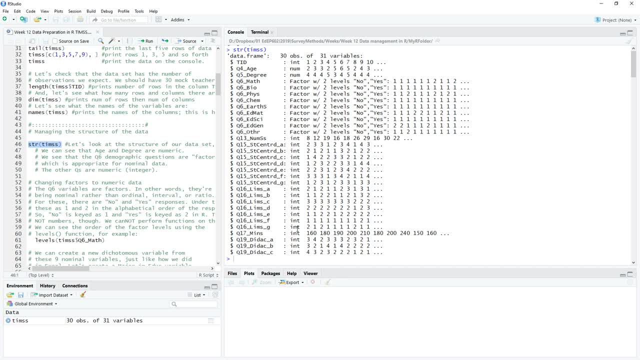 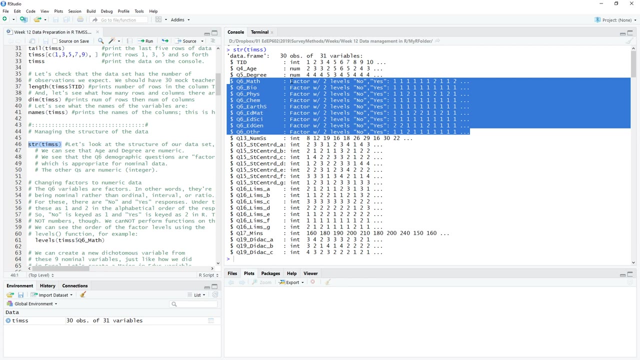 But these others are integer numeric, which means they aren't, you know, encoded with decimal places, probably because in the CSV file they were just whole numbers. And for question six, which is all of the demographics, they're read in as factor variables. 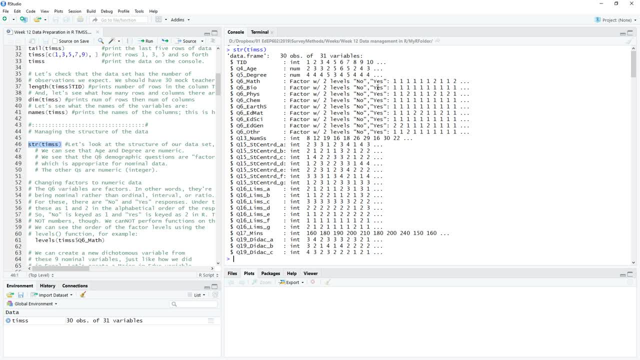 because the responses were yes and no, because some people had no and some people had yes. R interpreted it as factor So and it codes these under the hood in alphabetical order as one and two. So a no would be coded as one And a yes would be coded as two. 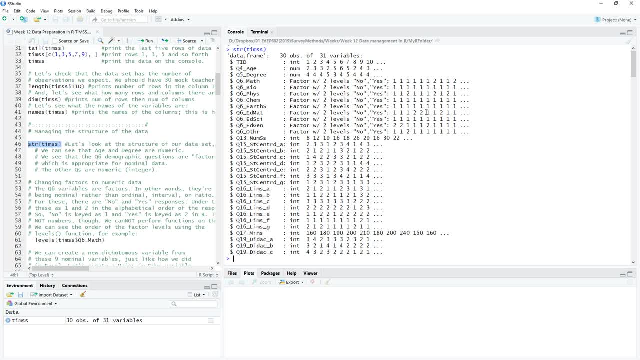 But when you look at the data, you actually see the yes and the no, And these are not numeric data. You cannot perform operations on them, But we can transform those into numeric data. So let's see, We can look at the specific levels of that factor. 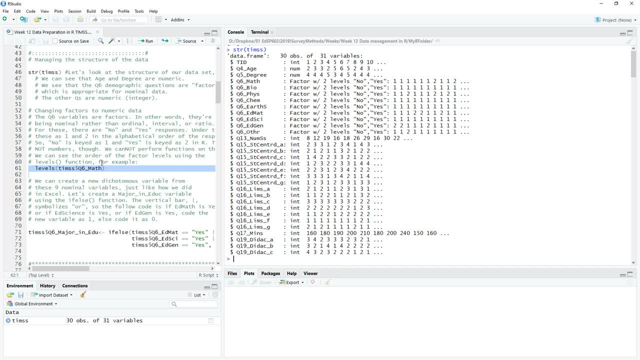 So these factors. let me look at Q6 math And I can see that, yeah, it is coded as no and yes, And the first one is one And the second one is two. We can change those as well later on, but that's in a different session. 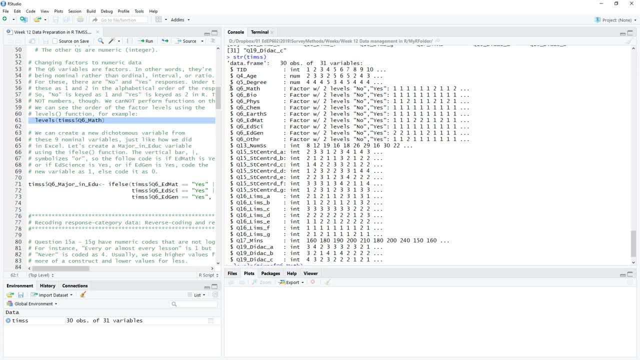 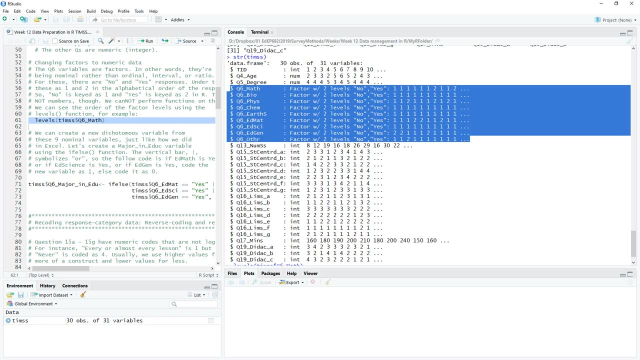 Let's see. Here's what I want to do. I've got these demographic variables of people's majors right. They could have majored in mathematics or biology or chemistry. In fact, let me pull up that TIMSS PDF. And indeed, yeah, it's asking during your college or university education. 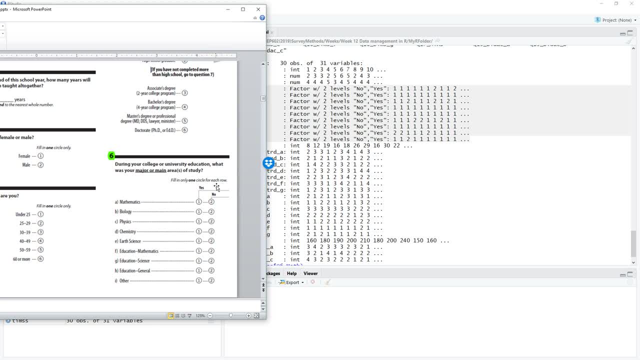 what was your major or main area of study? Fill in only one circle for each row. I like this question because it's yes or no instead of check all to apply, But anyway. so what we want to do is create a variable that codes these teachers whether they had 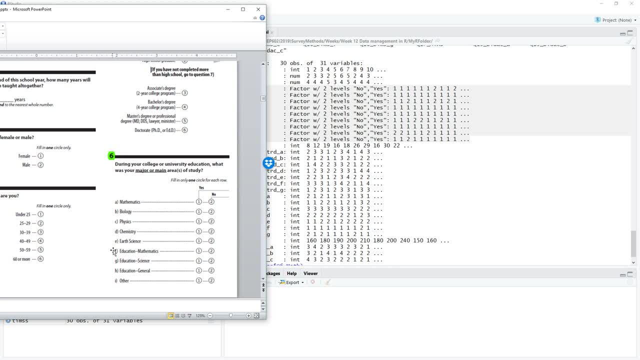 a degree in education or not a degree in education. So I want any teacher who has said yes to education, mathematics or science or general to be coded as one in my new data, my new variable, And any teacher who has no answer to that question, I want them to be coded as one. 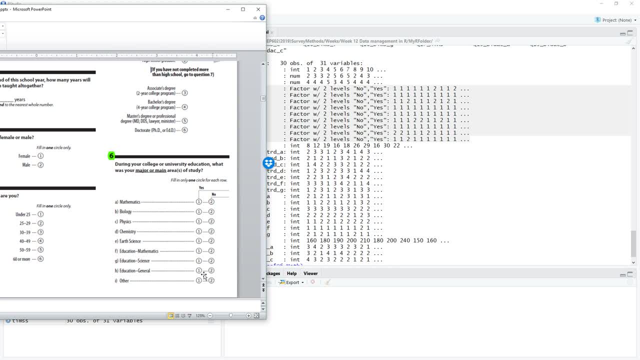 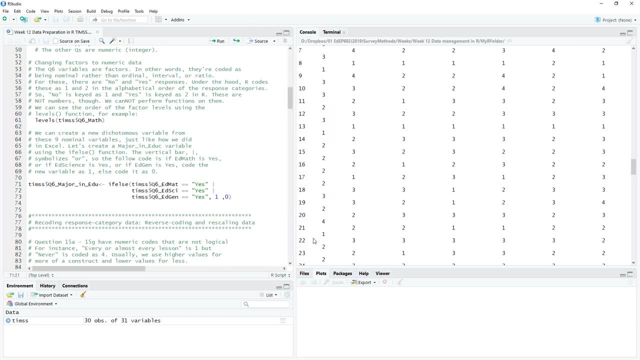 Any teacher who has not has said no to all of these or has missing data on these to be coded as zero. That's my new dummy variable, So let's look at the code for that. Basically, I can use the. if else function. 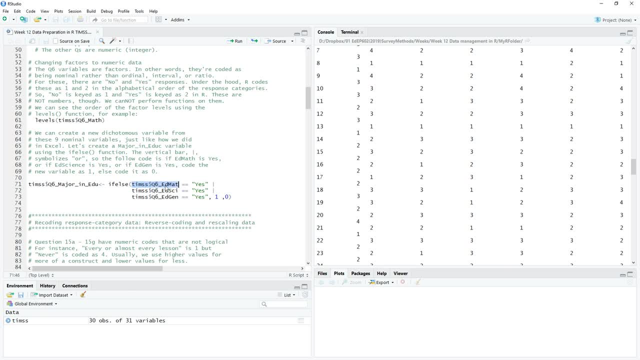 And so I say: if their score on ed math or their response on ed math is equal to yes, or if their score on ed sci, if they- this is just the name of the variable in my data set- is yes, or if their response to that third one, general education, was yes, then please code it as one. 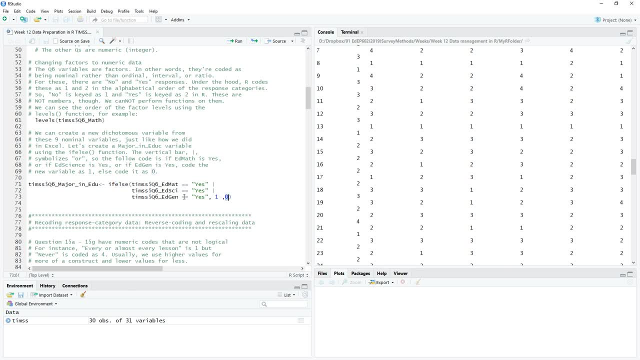 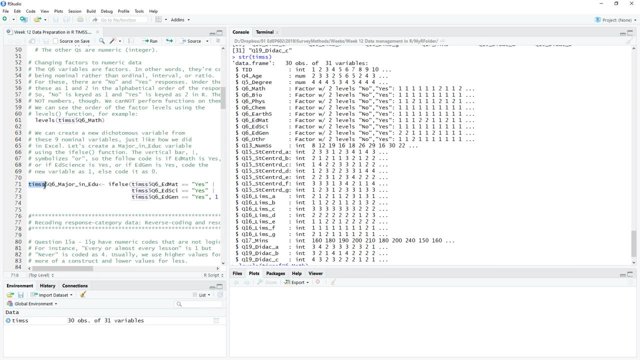 Otherwise, in other words the else. please code it as zero. So this will create a new variable and attach it to my TIMS data set at the very end. So if I look at my TIMS data set now, I don't see it. 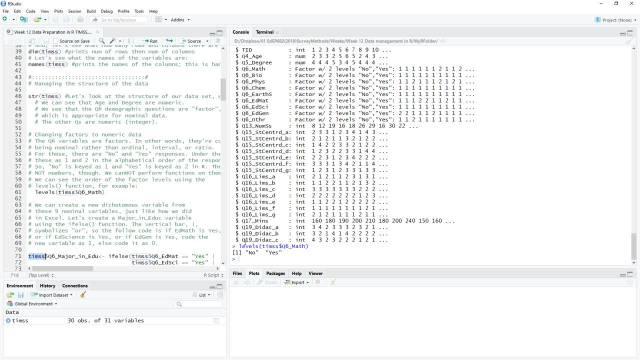 Like if I looked at the structure of TIMS, it's not listed, But in a minute, if I run this, I can see it. So if I run this line of code or right now, and then I look at the structure, 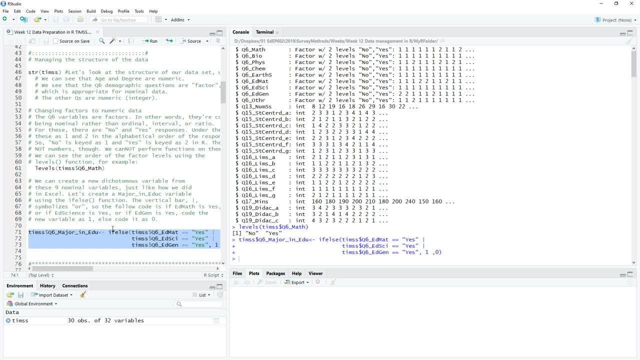 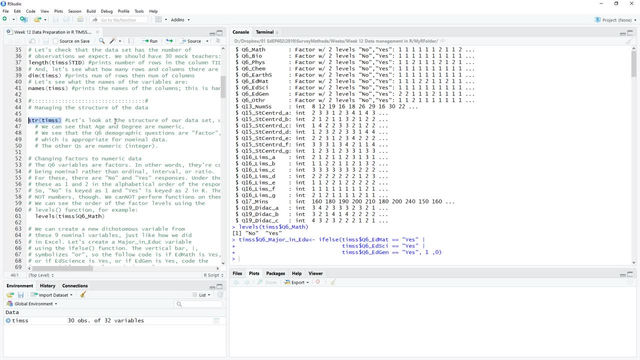 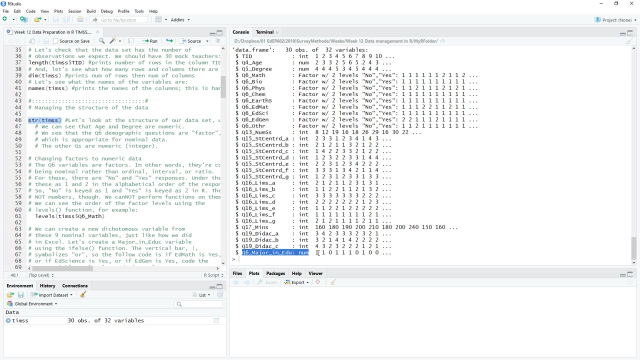 So I just ran this code. I used control enter, But you could also just highlight it and click run. And now, if we go up to structure TIMS, see, we have now our newly created variable. It's numeric and it's coded as ones and zeros. 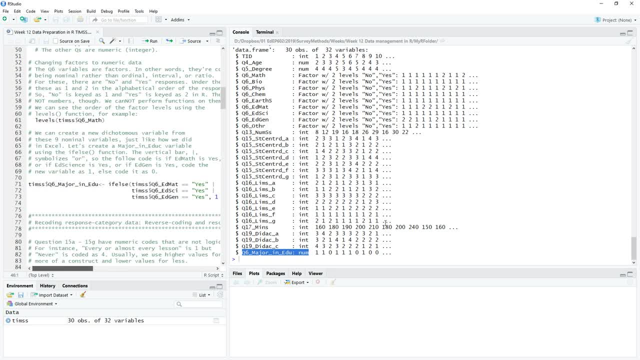 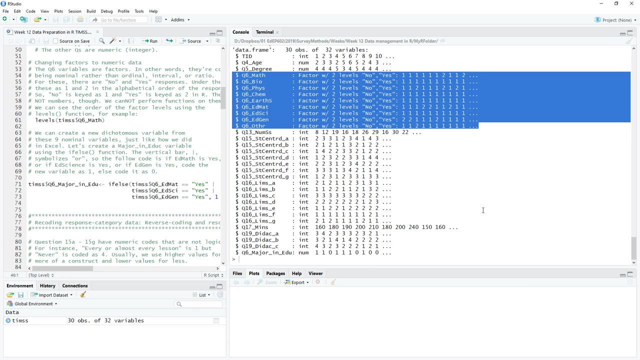 And I know what those mean because I just defined it. So this is a way to create a nominal or a new dummy variable based on lots of different nominal data, And this is very handy when we're going to use it in a regression, because we need enough responses in each category. 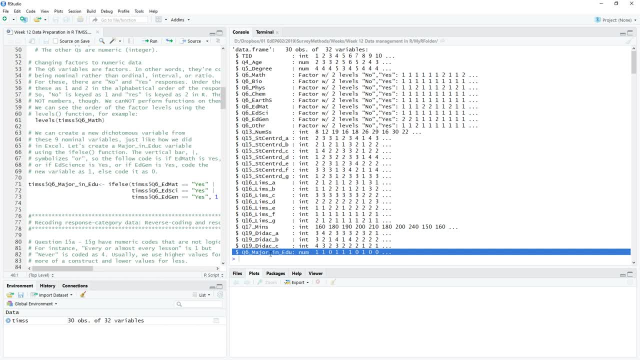 for these nominal data to function well in a regression. In other words, we won't have the statistical power to correctly estimate the differences between these numbers. So this gives us a very, very good idea of how the system operates. So this gives us a very, very good idea of how the system operates. 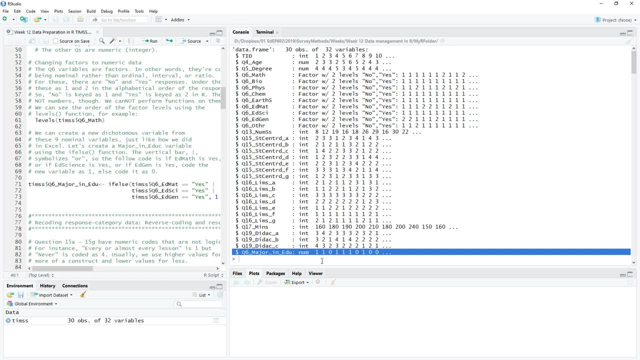 between you know two nominal scores, So collapsing them into a bigger nominal variable is really user-friendly when you do the analysis. In other words, this approach of taking several nominal variables and from them creating a dichotomous variable is valuable for addressing. 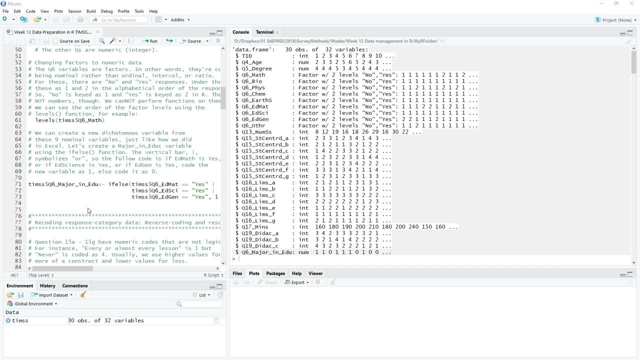 research questions that might ask about the difference between these types of teachers. For example, if our question were: what are the differences between teachers who have their degree in education versus those who do not, on a certain composite score that we're going to look at, such as their beliefs about how much learning should be student-centered in the classroom? 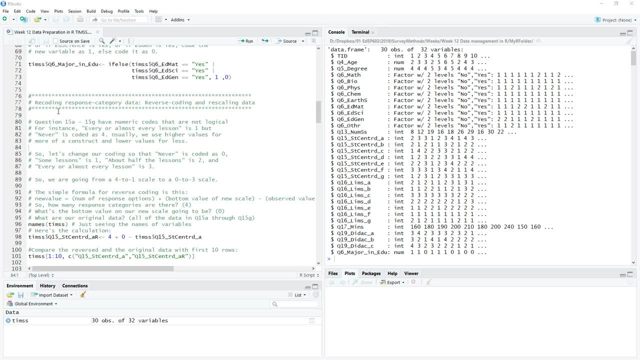 Next let's look at recoding response category data. First we'll look at- well, we will look at- reverse coding and rescaling data, actually both of those for question 15.. So look at question 15.. It has: the data are numerically coded but their order is not logical. For instance, 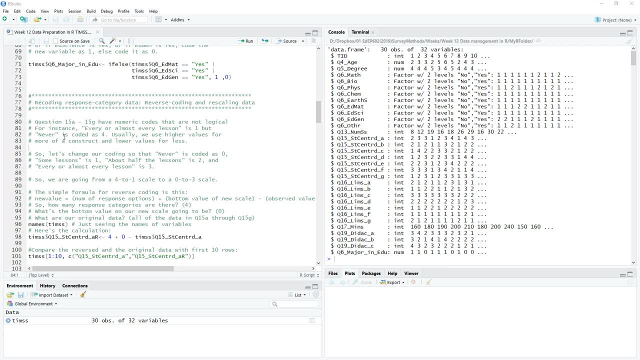 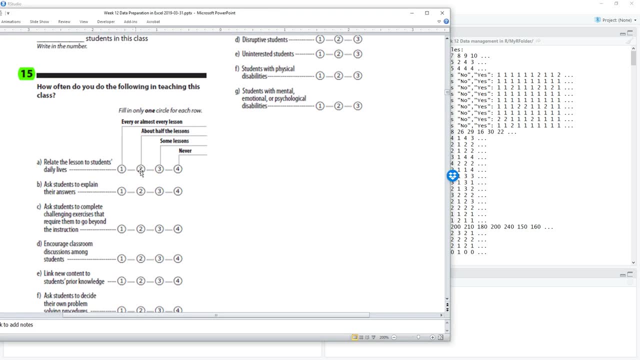 every or almost every lesson is coded as one, but never is coded as four, And this is because, Igor, our data entry person, you just used the codes that were in the instrument And so you can see if something is every or almost every lesson it's a low number And if something is, 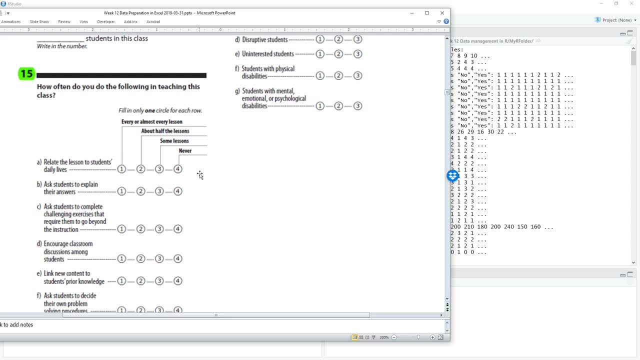 never. it's a high number. Well, that that kind of is contrary to the way we think about magnitude of a concept. So let's recode this so that never is zero. Some lessons is one, about half lessons is two, So that'll be the same, And every or almost. 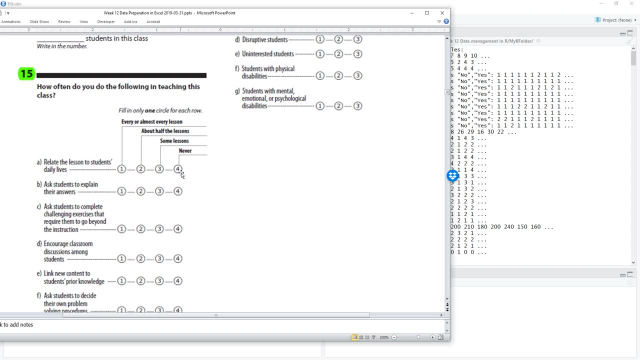 every lesson is three. I like to code it with a zero because that gives meaning to the intercept when we do analyze them. For example, if we were to use this as a predictor in a regression, although this would probably be the outcome variable. 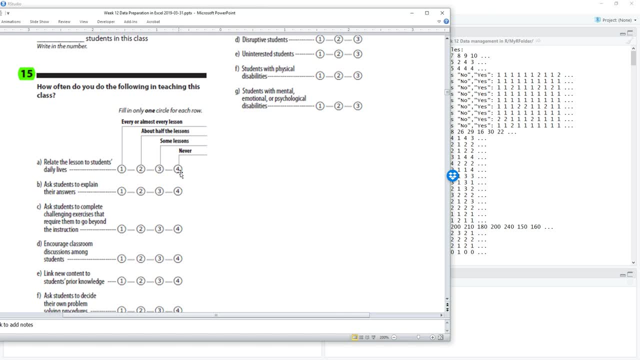 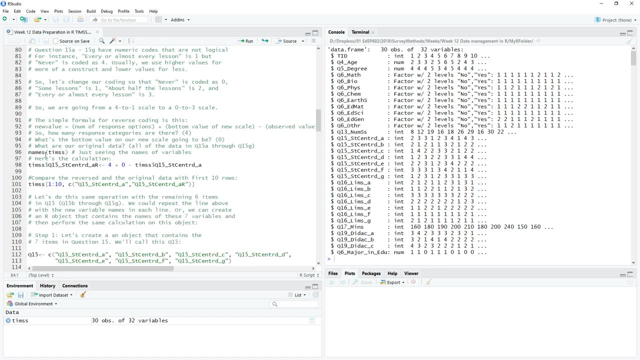 in a regression? it depends. Still, I just think it's valuable to have a zero. So if we go to our, our code, we can see how have I done this, If I, if I just look at the names of those, 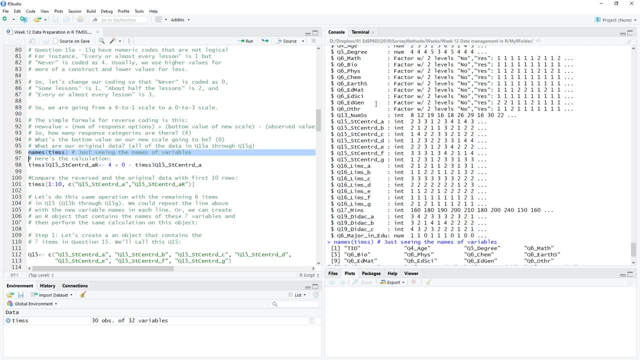 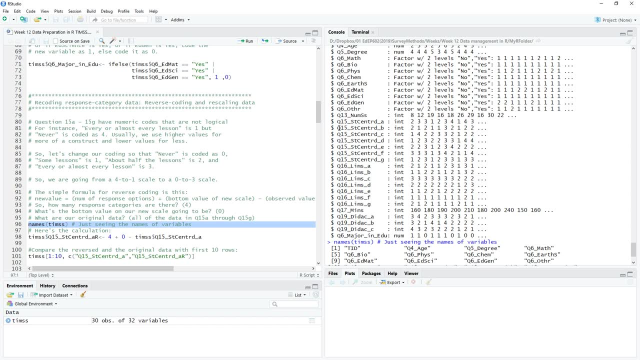 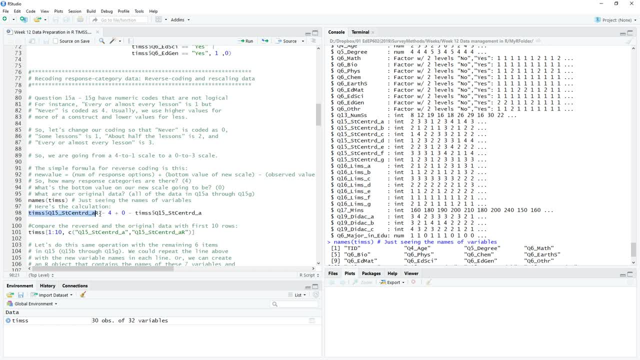 coded variable that is based on the original variable. I notice I just added an R to the end of it. so I'm creating a new variable, appending it to my Tim's data set and I'm performing the function, for which is the number of categories. I have right, I have four categories here: subtract or add zero. well, that doesn't. 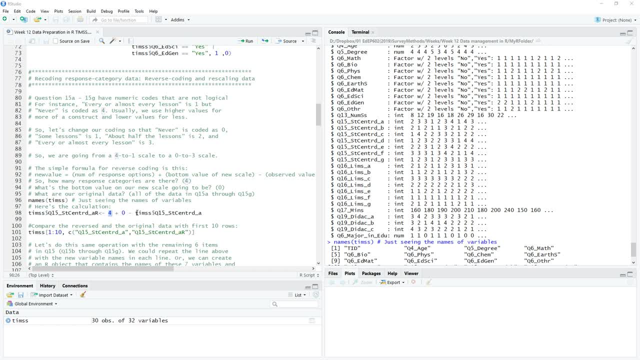 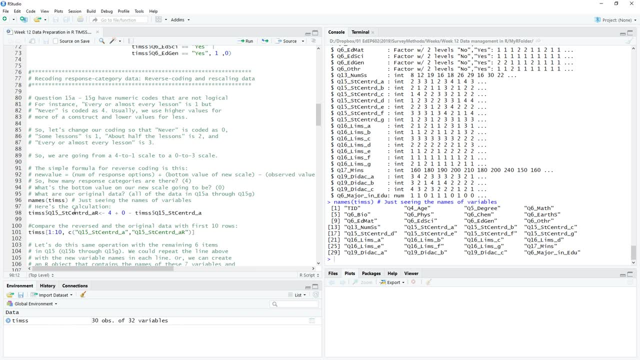 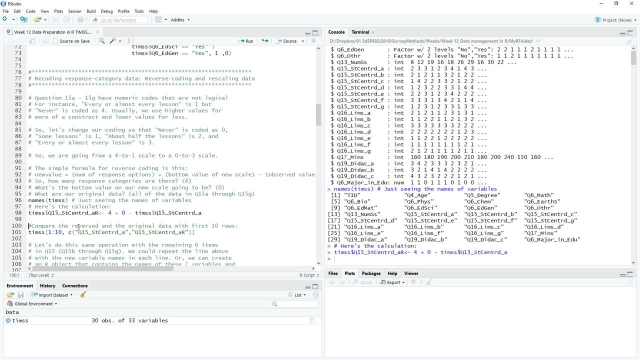 mean anything here, but that's the lowest value on my new scale and I subtract from that sum the present score of each person. and let's see, so if I were to do that, and I'm assigning that to the variable and now I can, I can look at if 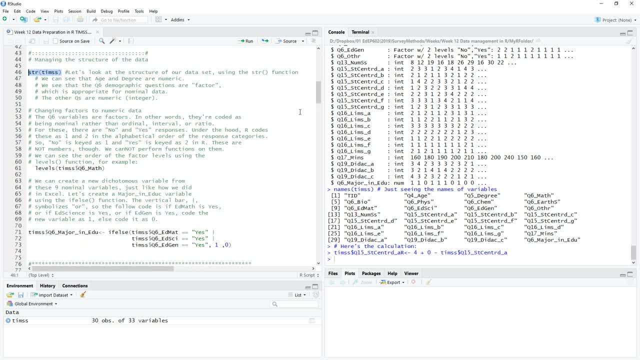 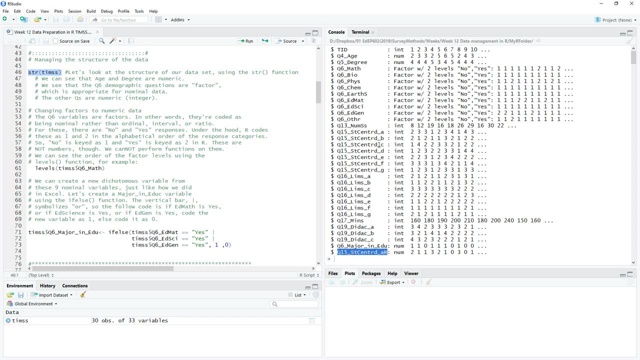 I did the structure again. I can see that that that new variable will be at the very end: q15: students centered a capital R. R is four reversed for me. I just put that in and here's the original one. so let's compare these two. in fact, you could even just look at the structure here and you can. 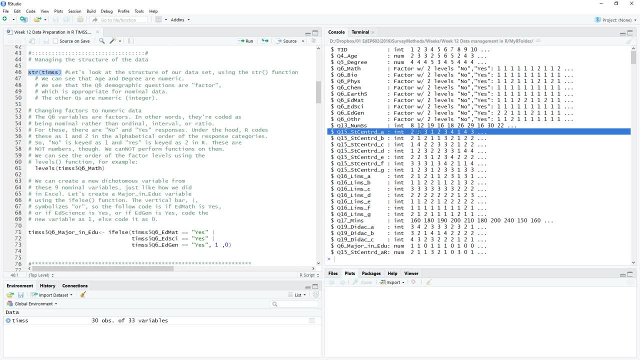 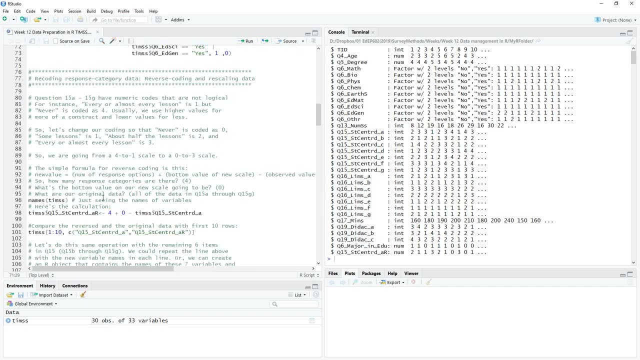 see well, person one scored a two, person two scored a three, person three a three and so forth on the original scale. but now it's a two for person one, a one for person two and a one for person three. we could also go back and actually just 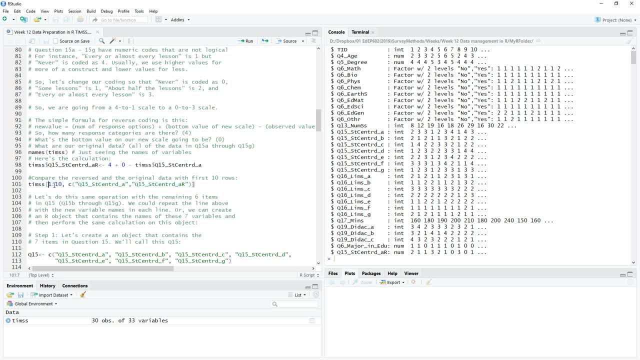 recall the first ten and you can see that here it's this kind of descending thing. so this is the first ten rows. so this is- I'm just calling up the first ten rows. and I want to get these two variables. because they are variable names, I have to include them in. 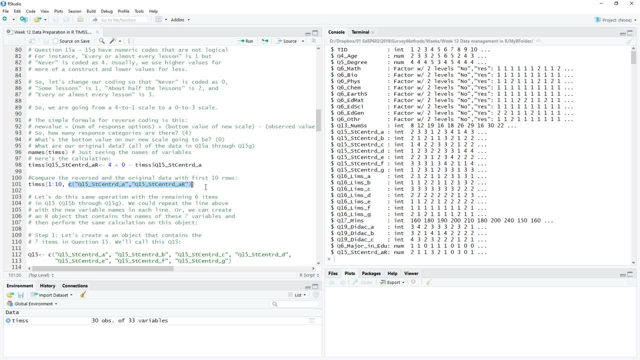 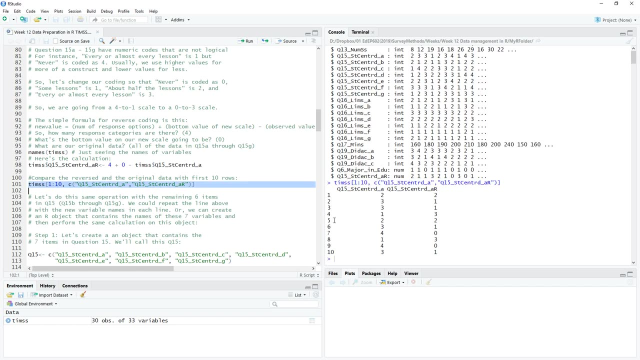 quotes and I have to include them also in a concatenate function, which is this whole thing, since I want to compare them. so this is an index notation, if you recall from the previous our session that we that we did earlier in the course, so, and you can see for the first 10 people, um, here are. here are the. here's the original response. 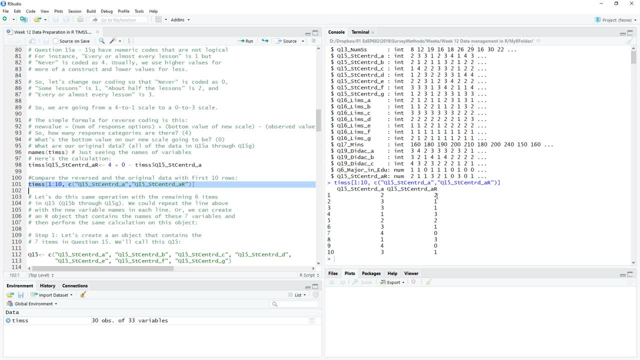 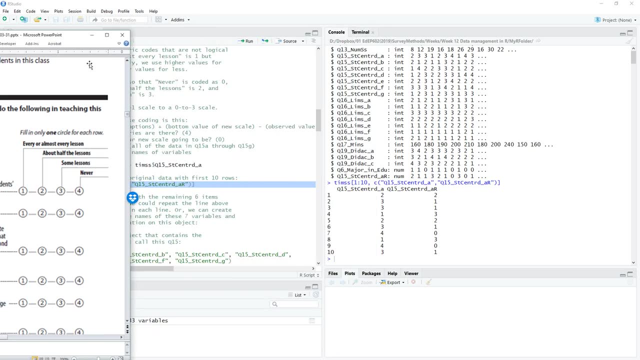 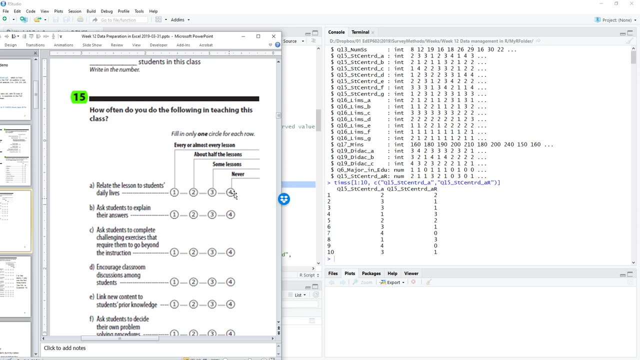 on that question. and here is the reverse coded: one. and, as i said before, two would be the same. so let's look at that. um, if i can pull this over, squeeze this in: yeah, so if somebody answered a two first person, yeah, that's answer to two, because i said zero, one, two, three, okay, so that two makes. 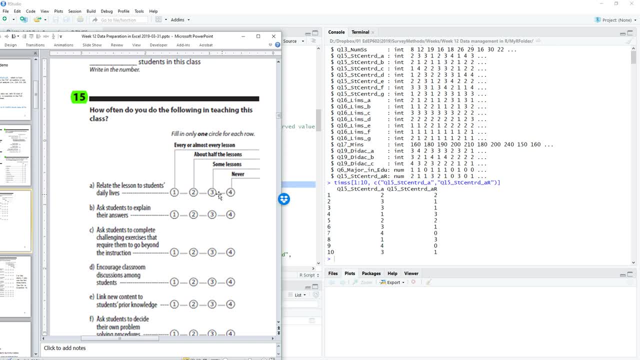 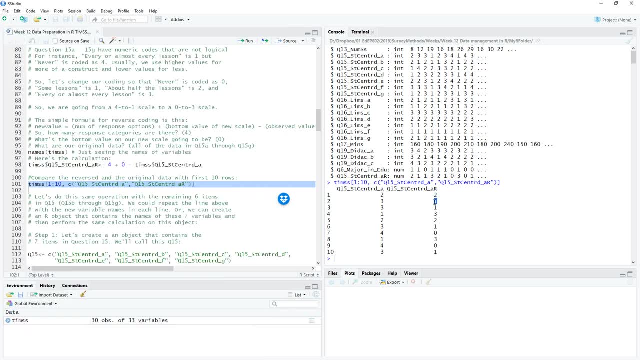 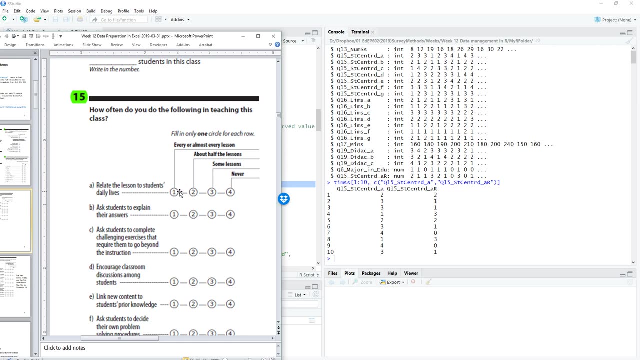 sense. uh, some, but this person answered a three, so that was the original one, but i want that to be: uh, a one, right, because it's zero. one, two, three, and is that? yes, that is indeed what i want. uh, and again the same for that next person. this person answered a one, so they said every lesson, or almost. 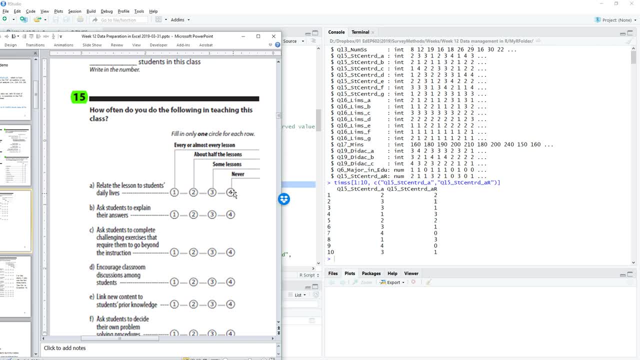 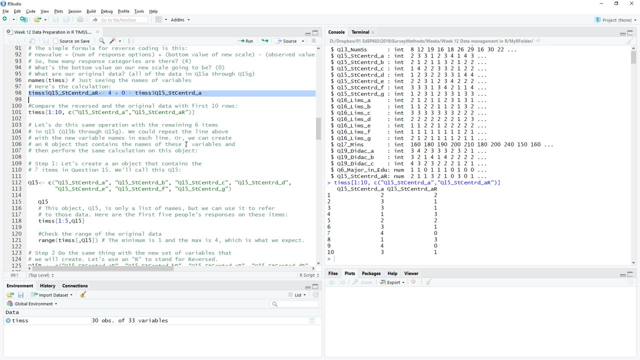 every lesson and i want that to be coded as three, because i'm saying zero, one, two, three, and is that what happens? yes, it looks like. uh, my function is working in the way i. i hoped it to. all right, so we could do the same operation with the rest of the uh six items. so i could you know? 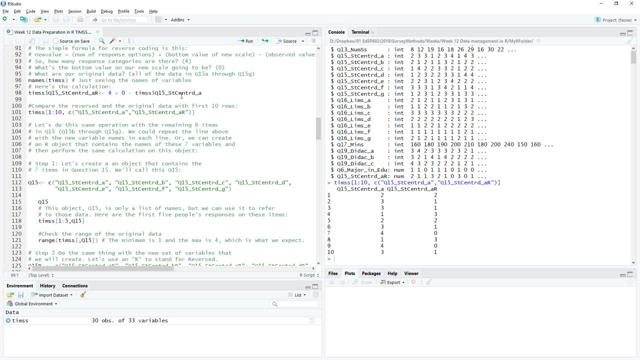 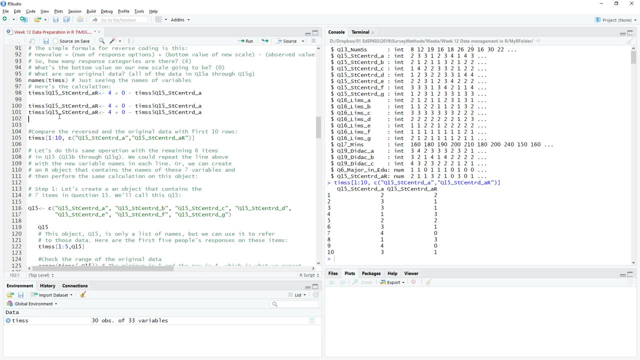 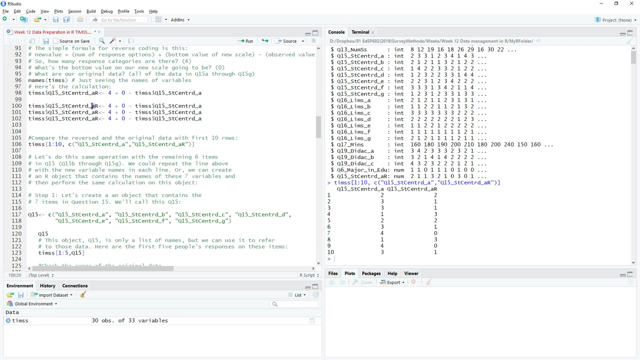 i could copy this line of code. i'm not gonna do, i'm not gonna follow through with this. just show you how i would do it. i would. maybe. i just took this line of code and copied it and then i'm pasting it here and i could paste it six more times and i could change this to b. 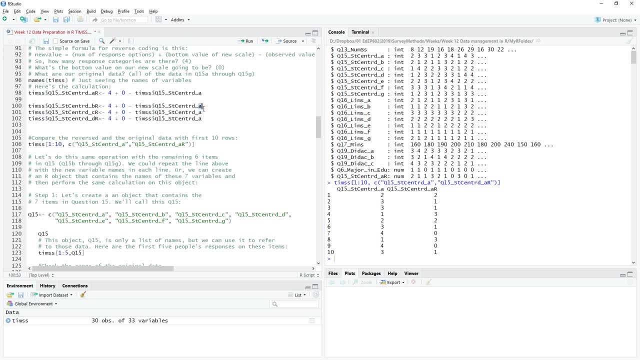 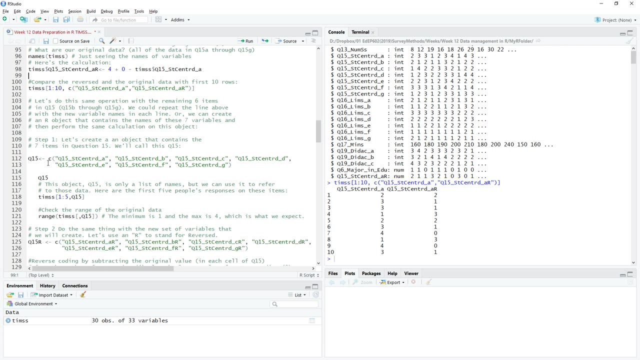 c, d, you know. so this is, this is kind of my workflow: b, c, d and so forth, all the way to g, and you would. you would get the reason if you ran those. you would um perform the same function on all of those. but i want to show you a different way, and that is we can create an object that includes the names. 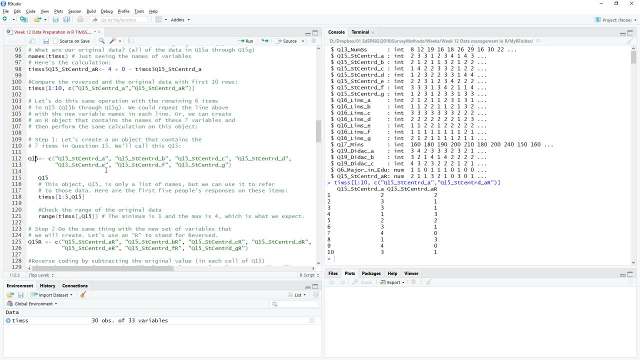 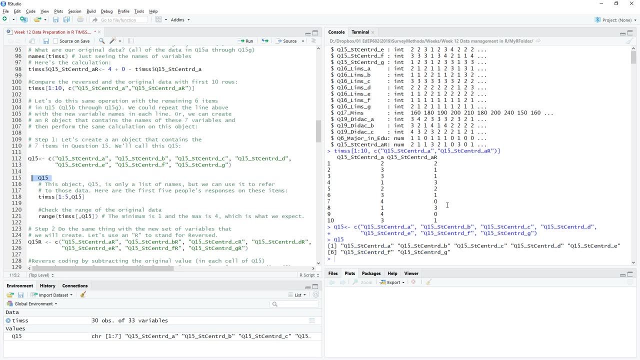 of all of the variables that we want to perform this function on, and i'll call it q15, and so if i i ran that now, if i actually look at that, you can see that it's just a list of all of the variables that we want to perform this function on. 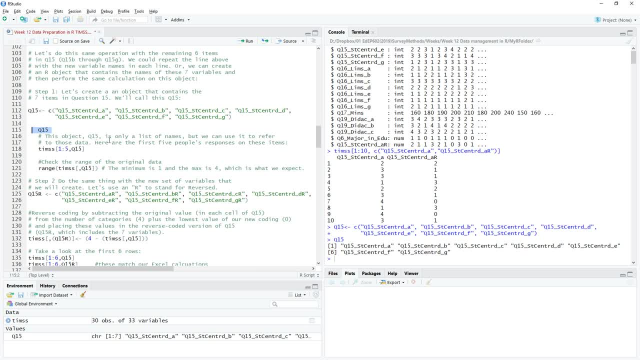 so it's just a list of all of the variables that we want to perform this function on, and i'll call it q15. so it is this, object q15. all it is is just a list of those names. it doesn't r doesn't know that that includes data yet, but we can use this list in our indexing to then say: give me those. 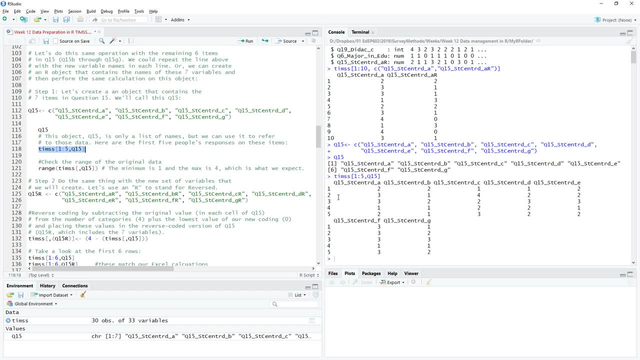 data. so here i'm asking for the first five rows of data for all of these, and i'm just going to place it in here, because what we're going to do is we need to find all of of the using army, and i'm then gonna show it to you in a second. 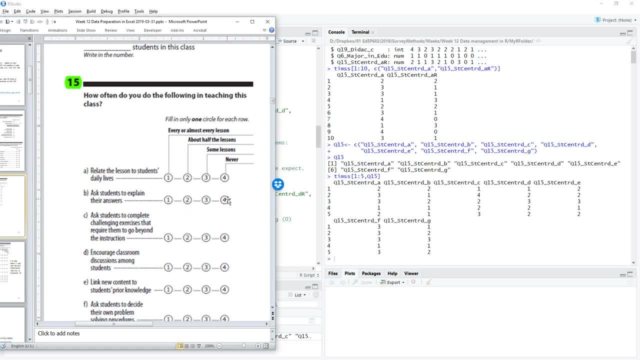 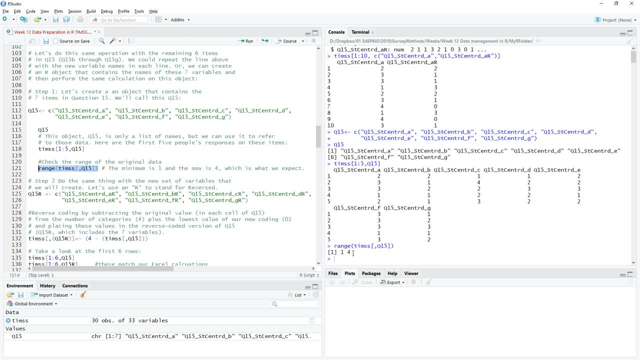 okay, if i can just turn this down, just just turn that off, that, for that's not a problem. let's. let's see people's scores. so the person who's been using q15 is somebody who types many times on the g world, for example, to get a phone number. so these two people here, so right now, if they start using this, 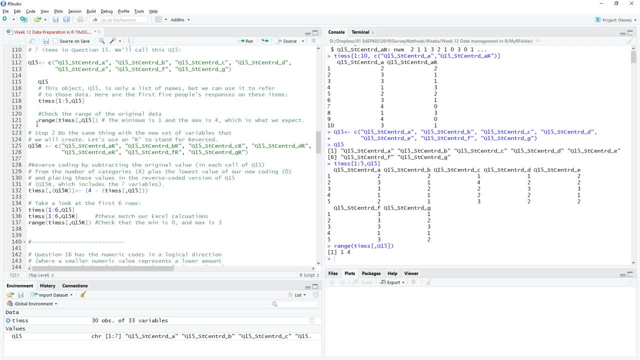 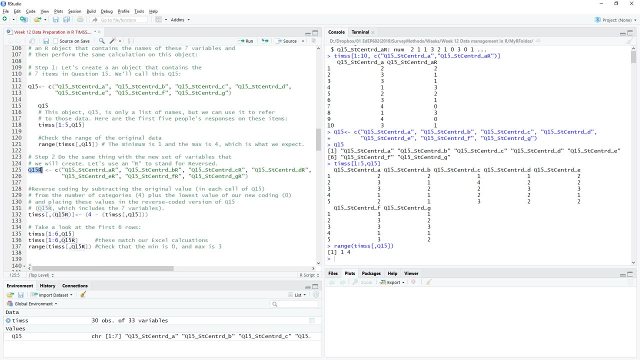 it's 4, 67 and if they start using q c, 15 on the g world or outside of the box. so these three are people who set a code and when they start using q c, c held on some simple, the same type of object. but I'm going to call it reversed with an R here and I'm just 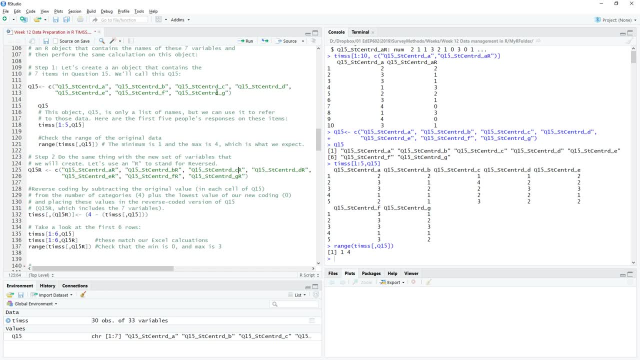 going to create these names with the Rs here. So I just basically I just copied this and then I pasted it here and I added R on the end of everything. And if I run that um, it will create a new object and again you can see it there. but 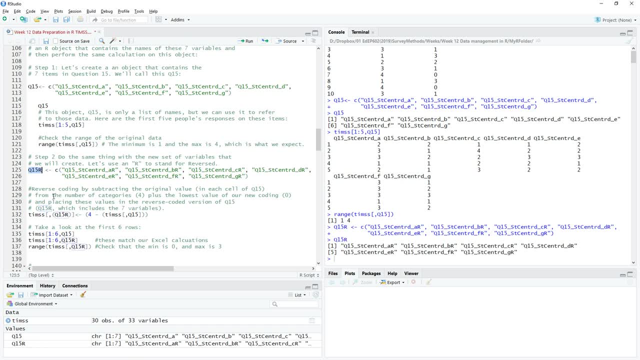 it's not in my data set, though. What I want to do is use this uh and attach it as new variables to my data set, So I use indexing, I use my Tim's data frame and the first before the um, before the comma. 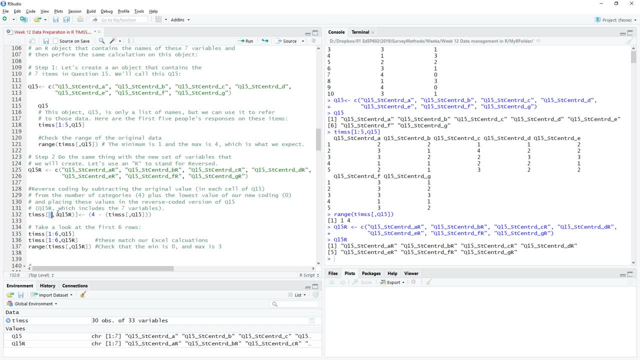 within the brackets is the rows, So I want this to apply to everybody. and um, oh, I don't know, I don't need this. um, parentheses here. And then the next is the object, which is: all of these things are. 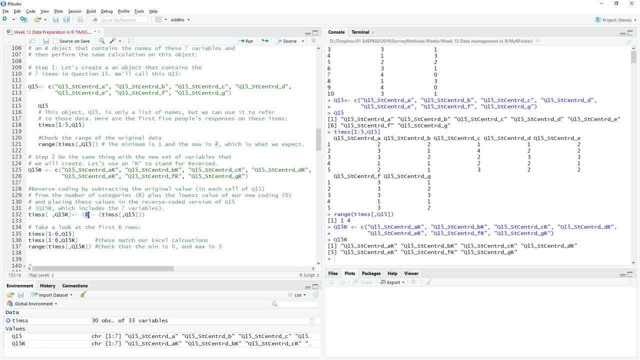 So I'm going to create this cause- the arrow is pointing to it, And here's my function: um, which is four minus. it's actually four plus zero, right, And then, And then minus: um- I don't need the parentheses here- minus the original data. 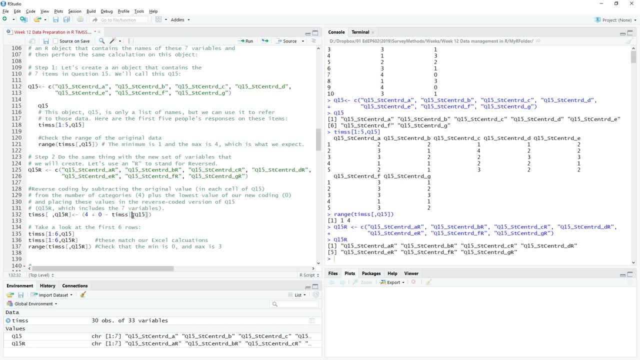 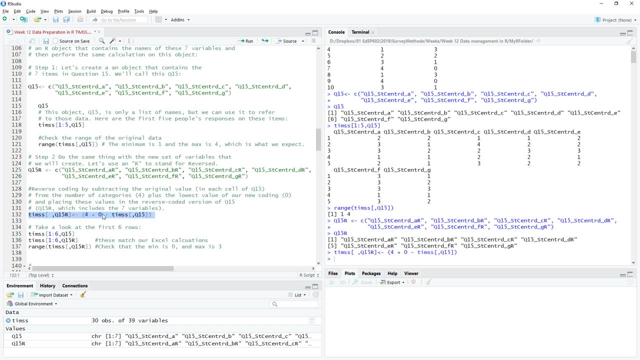 So here, here are the original data. yeah, for everybody. uh, with these objects that are captured in Q 15.. So I'm just performing a function across all the variables. Now, this would only make sense if they all were on the same scale. 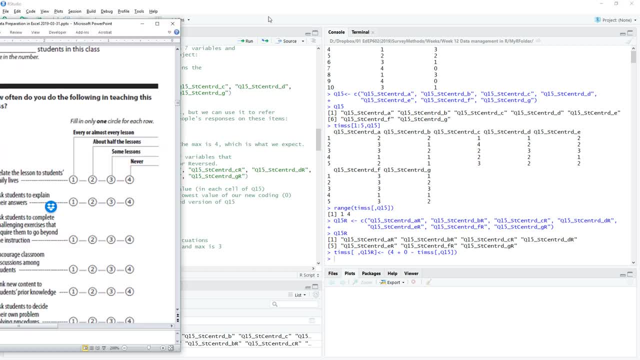 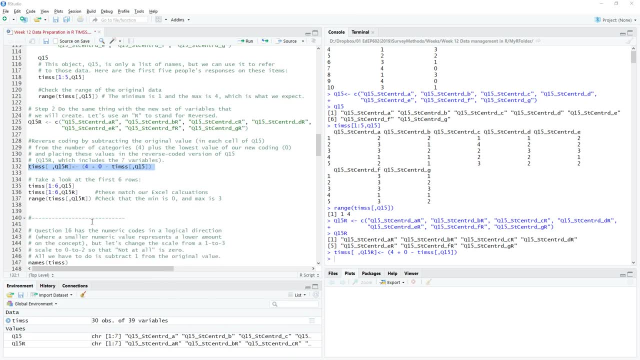 And in this case, all of them in question, 15- are on the same scale. If you look at, if you look at these items, they're all one to four. So now I'm putting them on zero. Zero to three. So let's take a look at our data. 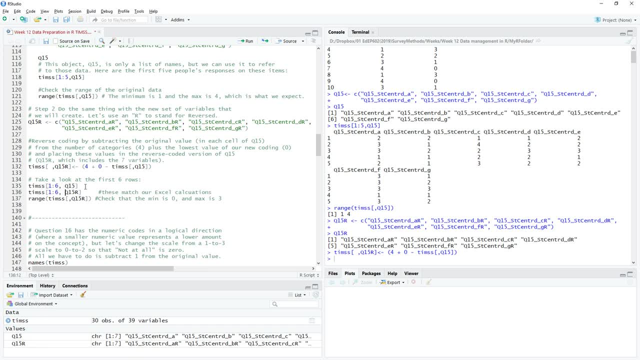 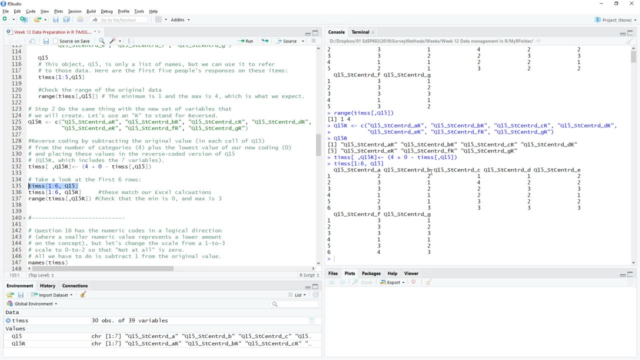 Maybe I'll look at the first six rows. It could be the first five, It's. it's really arbitrary, Um, so I run that, uh, and look, so the first six people I can see that, uh, that's the. 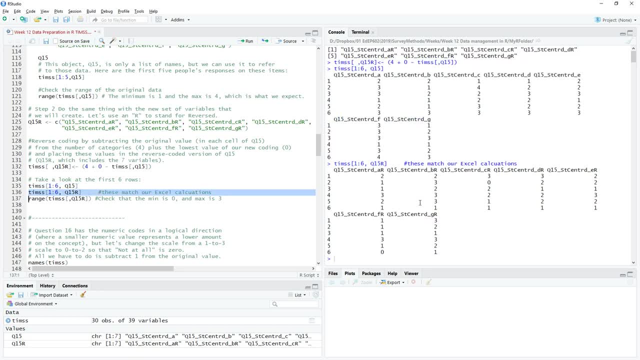 original data. Let me look at their uh reverse scores. and threes become ones, right, Uh ones, wait. threes become ones. Wait, threes become ones. Uh, ones become Threes. Yeah, Are there any four? 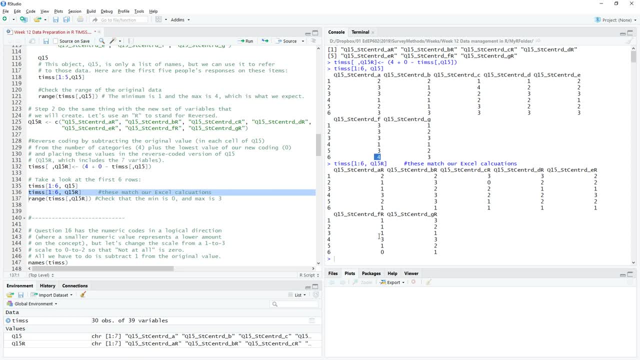 So here's a four, and the four became a zero here. So, anyway, this is a quick way to take a look at our data, and we can also look at the range of all of those data. What is the low and the high? And here the low is zero and the high is three, or the min and the max. 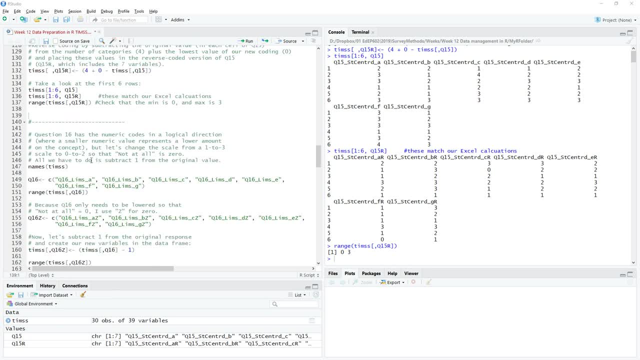 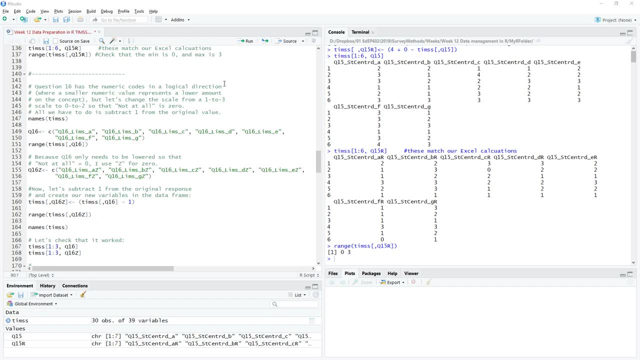 So, um, we can, we can see that that is what we expected. So we have successfully rescaled our data. Okay, From the zero to um three scale. And now let's look at question 16, uh, which has the numeric codes in a logical direction. 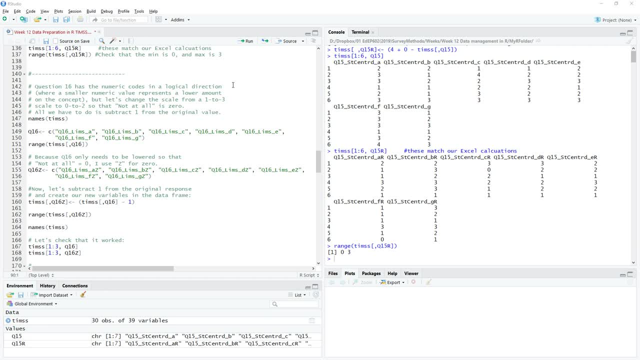 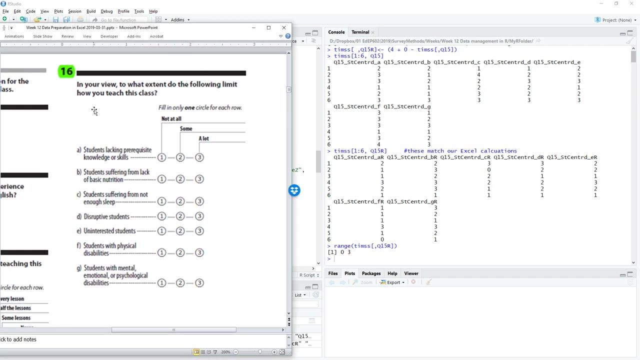 where a smaller numeric value represents a lower amount of the concept. But let's change the scale from a one to three scale to a zero to three, excuse me, to a zero to two scale, So that not at all is zero. So here is the question: in your view, to what extent to the following limit? how you teach. 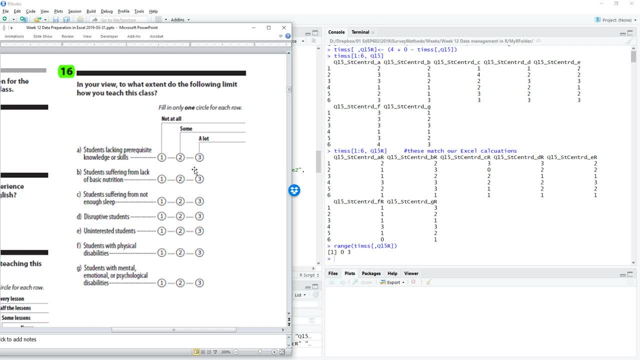 this class- Okay, Not at all- is a low value and a lot is a high value on the original scale. Ah, I like that. That's good, Thank you, But um, I also like to have my lower number be zero. uh, zero one and two. 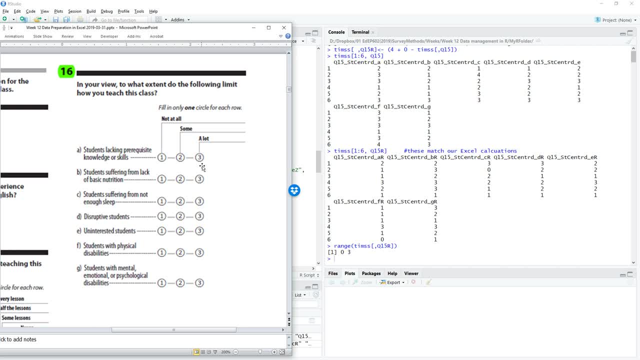 So if I put it into a regression or if I take the mean um, then it is on a scale from zero to two. Uh, you don't have to do this, and a lot of uh researchers just stick with the one to. 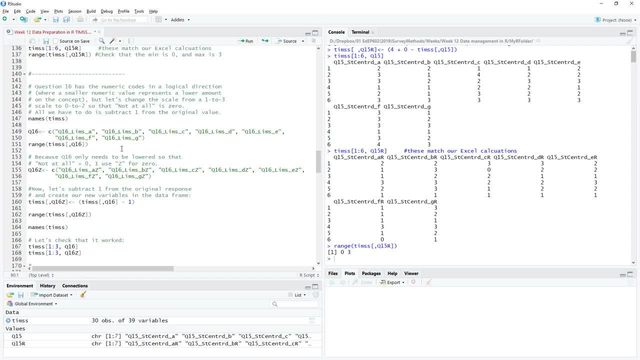 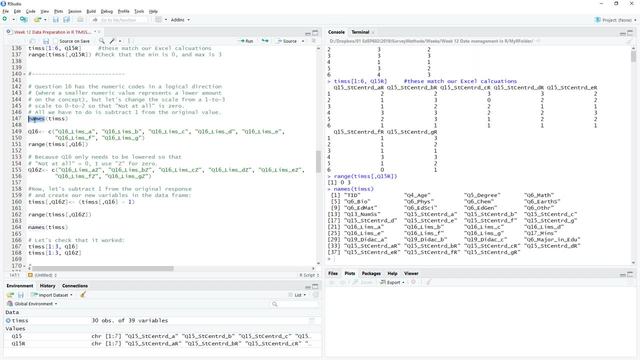 three scale, but I'll show you how to do it anyway. So, um, again, I want to make sure. Um, again, I want to make sure I get the names of my variables correct. Um, I could also use the structure or the names and look at all of my data. 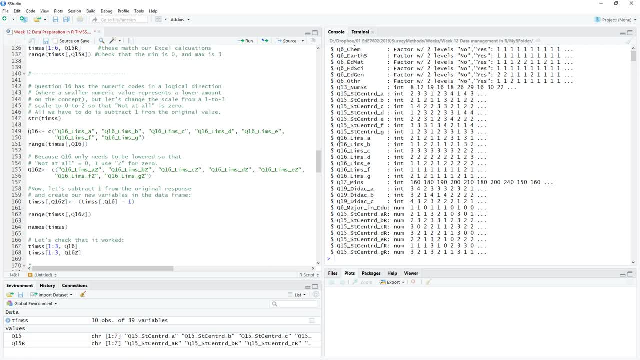 Let's see. So I'm interested in Q 16, right? So it looks like I'm labeling them limits or limbs. uh, Q 16: limbs a, B, C and so forth, all the way to G, And it looks like they are on that one to three scale. 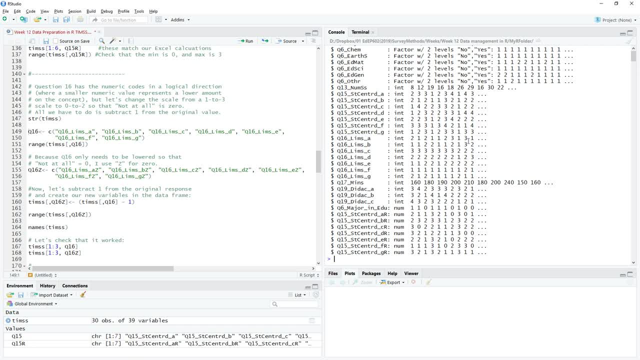 This is the first person, The second person, The third person And so forth. I think it's the first 10 data points. So, uh, again, I can assign all of these items. So basically here, all I did was just copied. yeah. 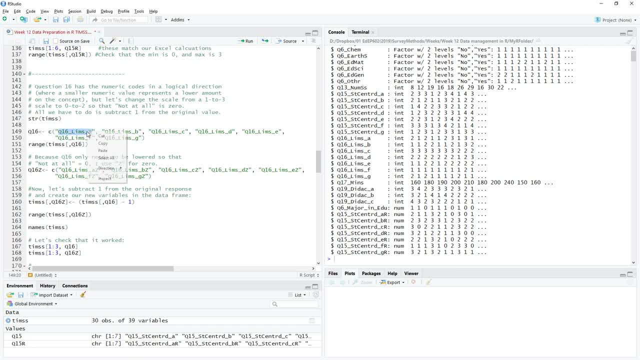 And pasted these and put quotes around them. Yeah, For everything. Actually, I just probably copied this and then changed the A to a B and the B to a C and so forth. Uh, but they have to have commas, Yeah. 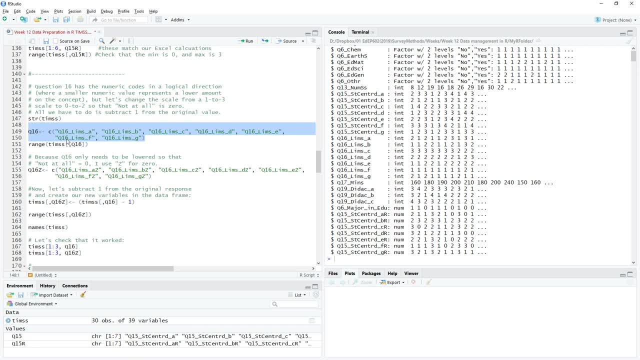 Between the, the quoted ones, The, the quoted um, Um names, then you can apply them to the object. So I run that and then I ask: okay, with my Tim's data, which is all, all rows and the. 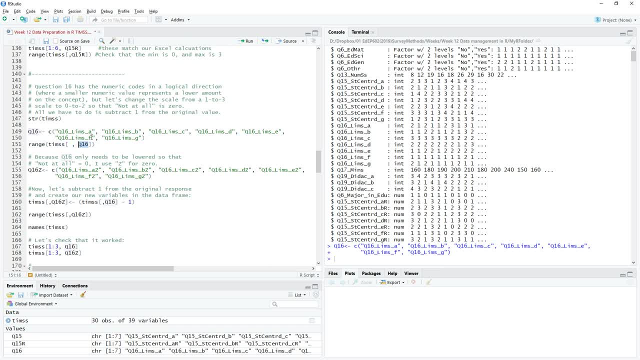 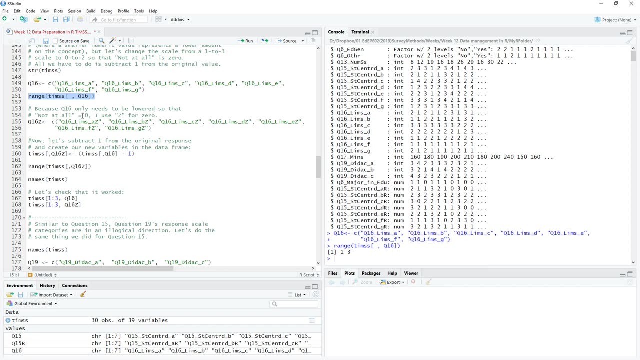 columns that are captured by all of the variable variables that are captured in this name. what is the range? And I think it's one, two, three. Yeah, The min is one and the max is three. And because question six only needs to be lowered, uh, so that, um, not at all, is equal. 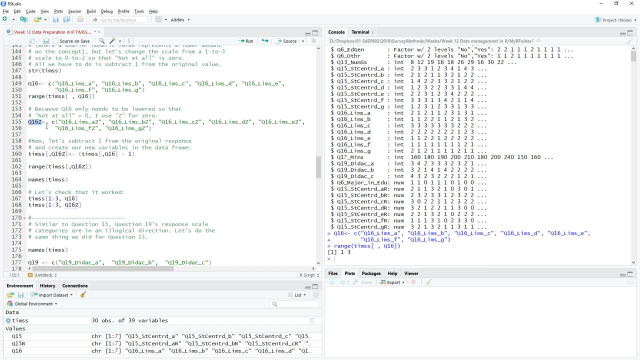 to zero. So I just added a Z for zero in my new variable name and I just added a Z. I just basically copied this line and then pasted it to this line and then added a Z behind everything. Um, this is a nice way to be sure you can track your, your data and we might not actually 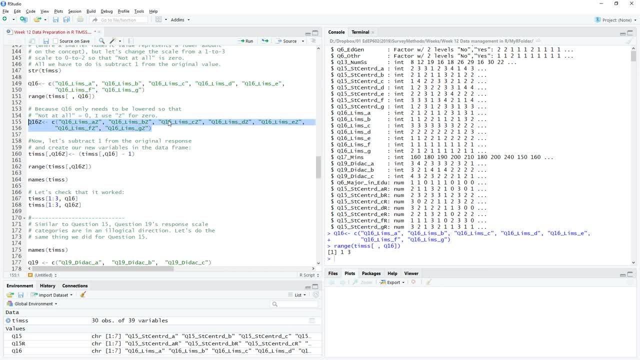 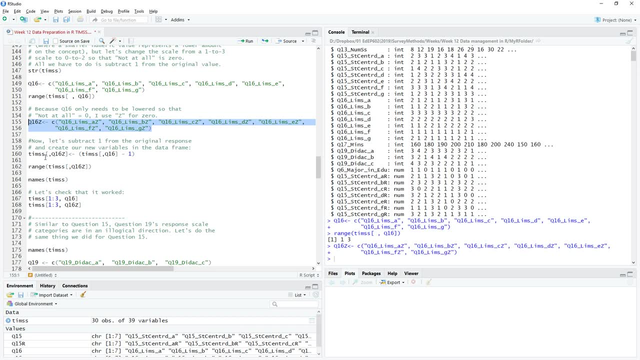 use these, but you know there's no limit to the number of variables as far as I know, that you can have in R. So it's it's good to do that. Um, so I have created my new variable. I can perform the function on it, which is for all of the Tim's data. uh, excuse me. 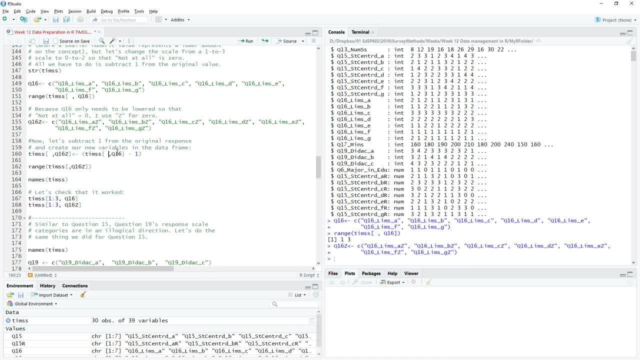 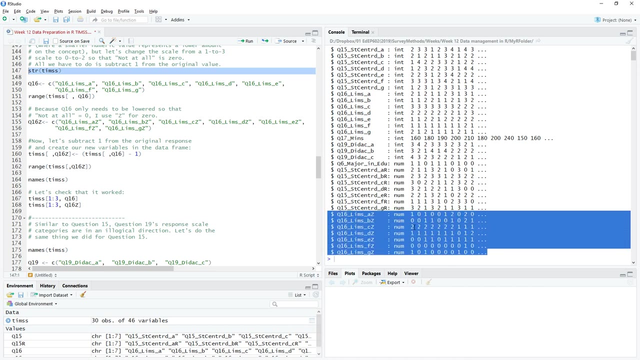 for all the Tim's data on Q 16, that is, for all of the rows, for all of these um variables. just subtract one and then assign that to a new set of variables. And now, if I look at the structure, I can see I have successfully created these data. 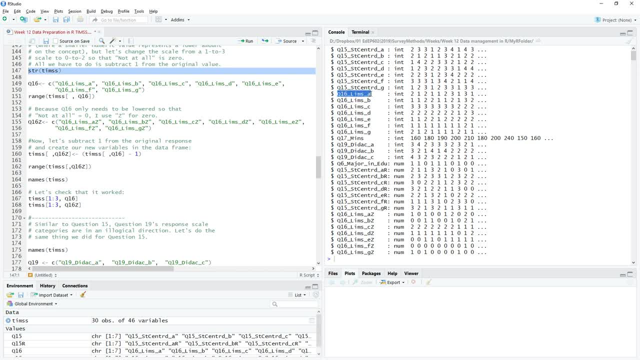 and I can see that. um, here's my Q 16 limbs a original. The first person had scored, It had responded with a two, the second person with a one And if I look at limbs, a four zero, it's again. obviously I have subtracted one from these. 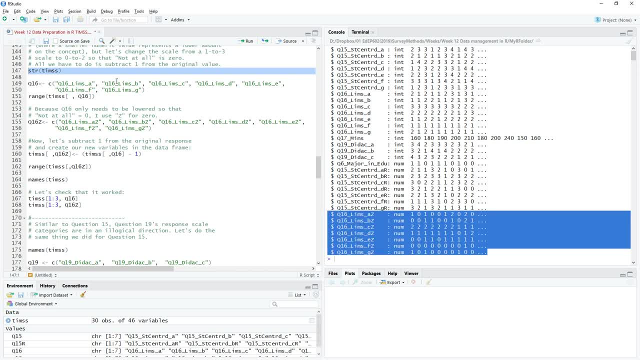 So you can see that the data um are correctly. it's always good to check, make sure that your calculation worked, uh, and that there are indeed data. So, uh, let's see I could look at the range. 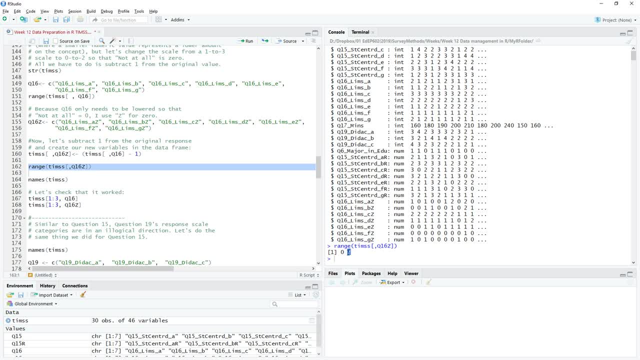 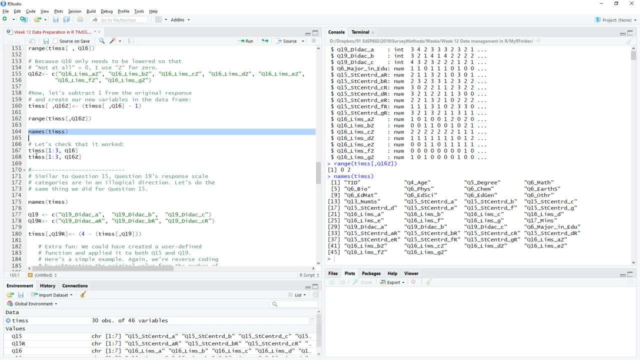 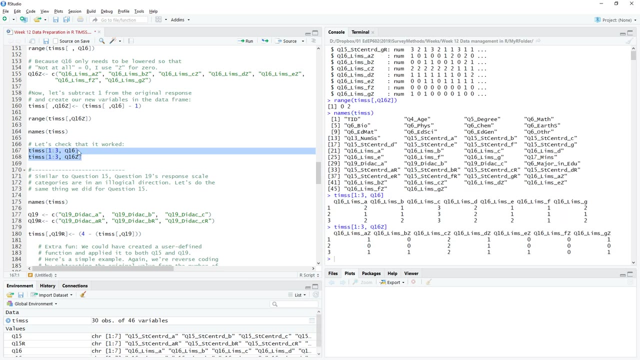 It should be from zero to two. Yeah, The min is zero and the max is two. Okay, Um, I could look at the names here. That's just to verify that those variables were created, And again I can look at how it worked by also just looking at the first three people. 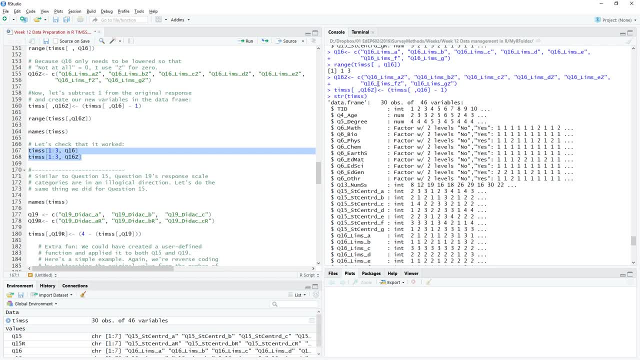 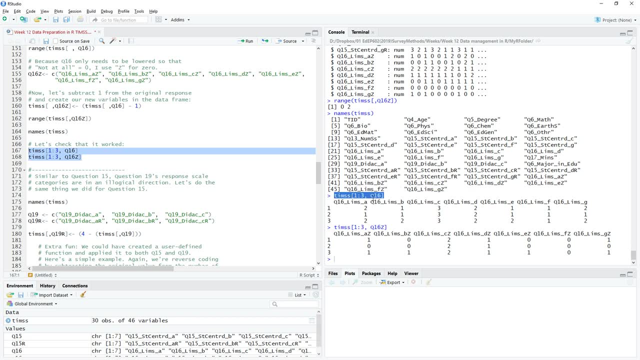 in this way up here I did it with a structure function, but, um, I could also just do it with this kind of function. or I just say, Hey, give me the first three people on on these, and give me the first three people on these, and I can eyeball them and see, okay, 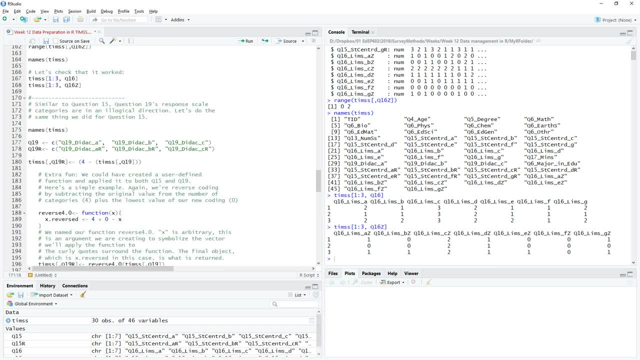 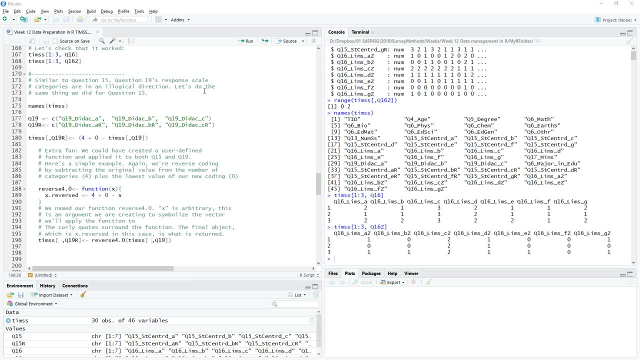 that does look correct. My calculation does. Question 19 is similar to question 15 and that its response scale categories are in an illogical direction, at least how they are numerically coded. So let's do the same thing that, um, we did with question 15 here, uh, with question 19.. 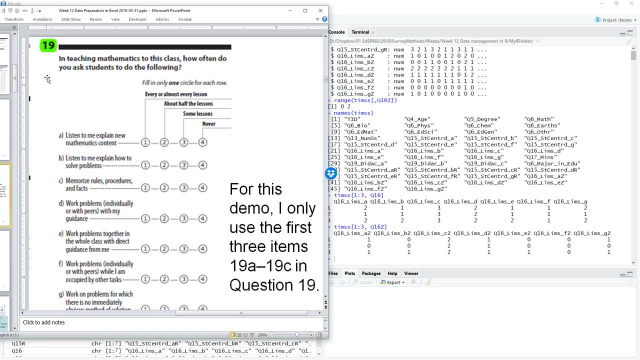 So here's question 19.. It asks about: in teaching mathematics, how often do you ask students to do the following? You know, listen to me Explain, Okay, So I want to. they have coded this as every or almost every lesson, as one, uh, the lower. 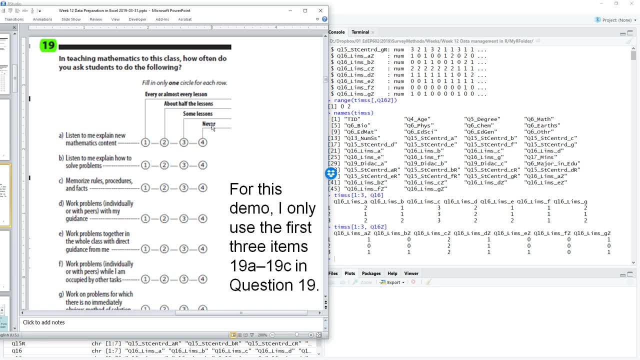 end of the scale and never as four as the higher end of the scale, And I prefer to have these as zero for never, one for some, two for about half and three for every or almost every lesson. That way I can interpret the scale, which is, you know, when I run a regression I would 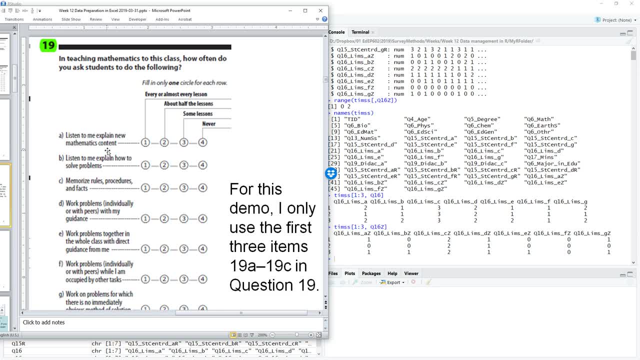 expect this to negative. So that would make sense if the scale is in the same direction as the concept. So I'm only going to look at a, B and C here, but we would do the same thing with all, all of these all the way through G. 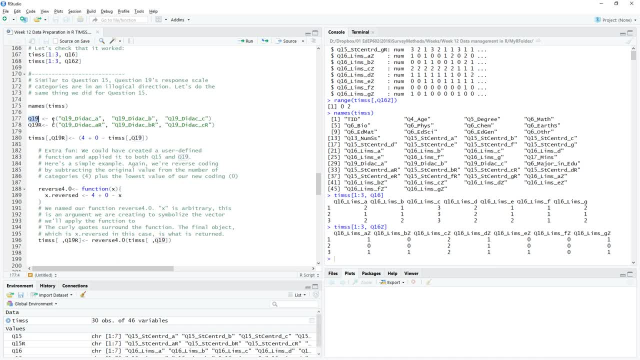 So the um. here again, I'm creating an object called arbitrarily- I'm calling it Q 19 for clear reasons, Um- and within this object I have the names of all of my variables. I could run the structure function too. 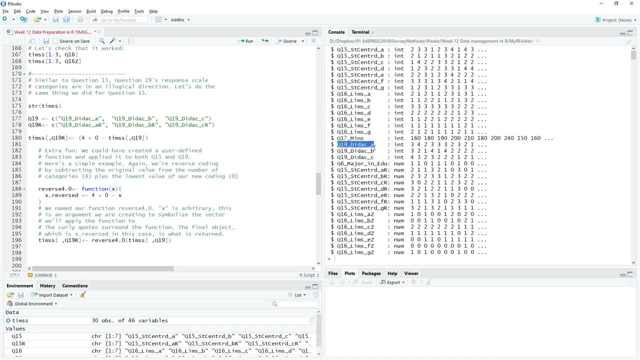 I could list them to make sure I have named them correctly. I might copy, yeah, copy that and paste it there. um, just to be sure that I have these names correct, Otherwise I will get an error. And um, then I'm creating another um object called the reverse of Q 19 or Q 19 R. 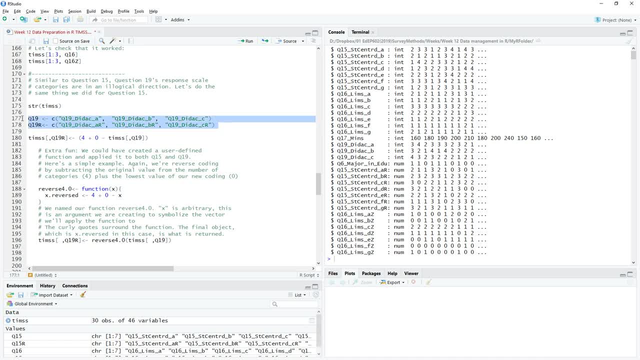 And I just added R to each of these. So I'm I'm creating these two objects and from 19, I will create 19 R, Uh, Using this function which is um, again, it's on a. there are four, four options and 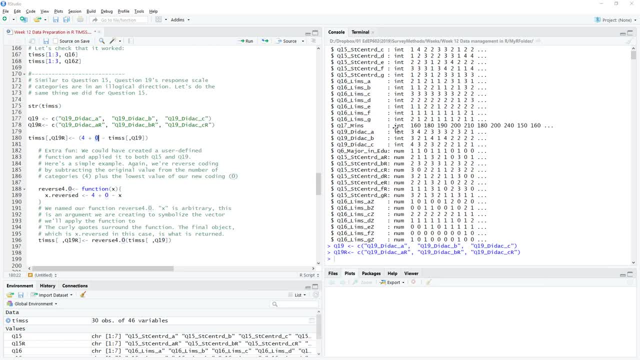 my new bottom of my scale will be zero. So I'm going to that's. so this actually just goes away, of course, And I want to subtract from that my original data. So, let's, that's how we would reverse code. Uh, so let's do that and I can run the structure function again. 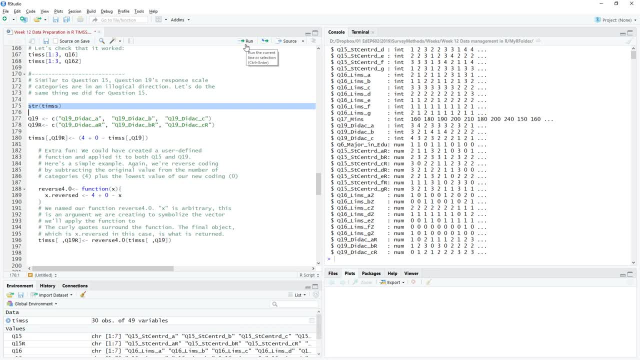 I've just went up here, selected that And I did control enter. You could, you could click on run And here we have Q 19 didact- AR, and Q 19 didact as in didactic teaching. yeah, A So person. 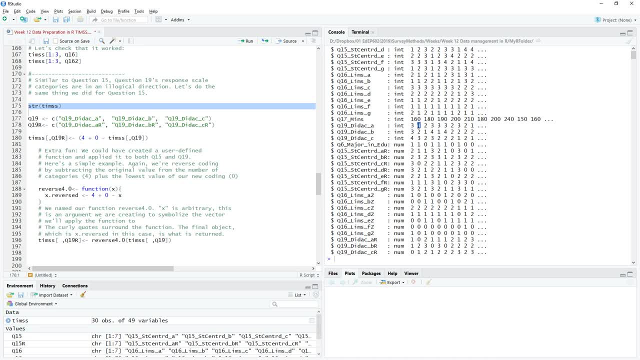 one teacher, one said three teacher, two said four teacher, three said two, and so forth. That's the raw data in the original set And if I go down to this one, it's it changed to one zero two, and so forth. 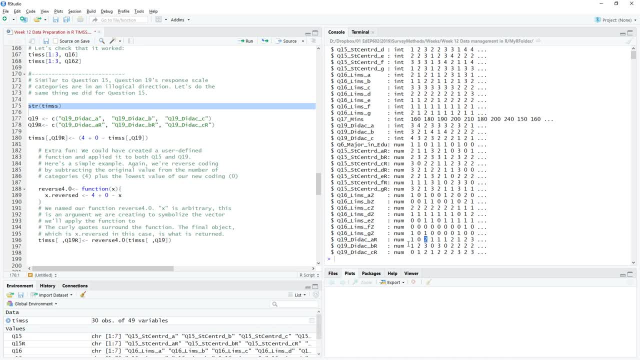 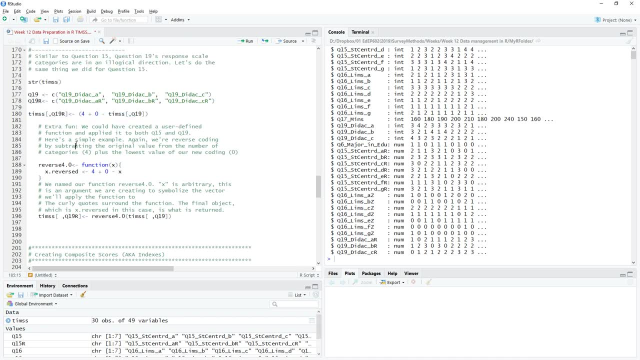 And and so you can check to be sure That that is indeed a reverse coded um. just as we did before. Here's some extra fun Um. I know you're always looking for fun stuff to do an R and I guess it's you know the. 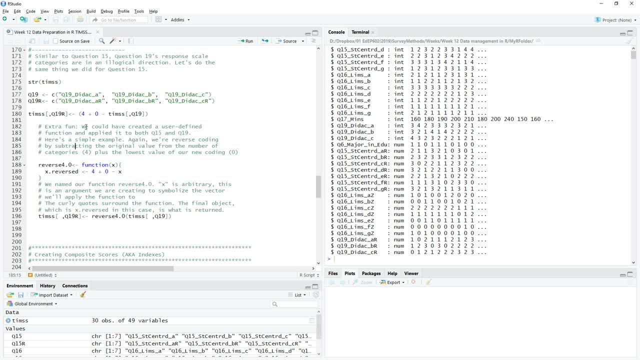 nerd alert time. but basically we one of the fun things in ours: we can create our own user defined functions and apply them to um to data. So because both question 15 and question 19 required the same type of function, 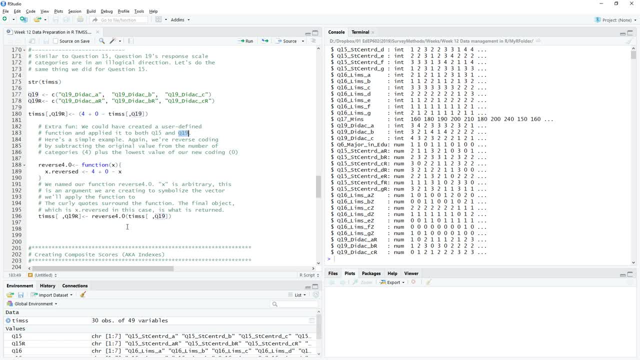 Why not create this very simple function and then just apply it? So here I'm just applying my newly defined function to my data and I'm going to create, uh, the new set of data. So this achieves the same thing as we did up here, but we could also use this function. 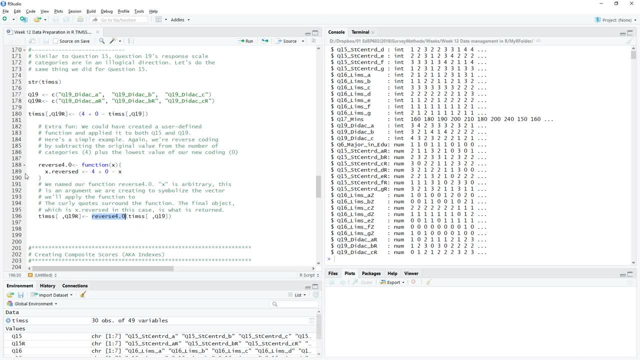 with other data. So if we have lots of similar data, we can do that. So here's how we create a function. First, we decide what our function name should be, And this is one- This is an arbitrary name that I just created called reverse 4.0, because I've got a four. 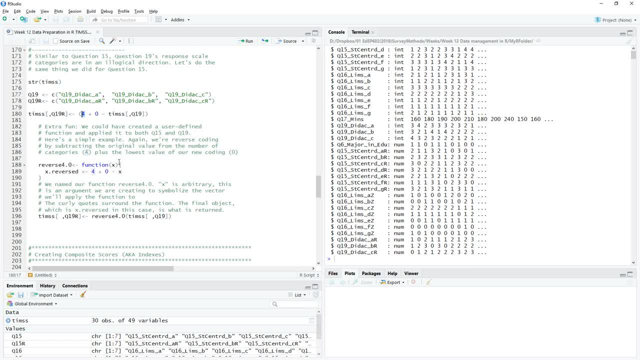 point scale and I want to reverse it. Um, you want to use names that are does not already have as a um, as a function, So you might check R by doing something like help and then put in your you know whatever. 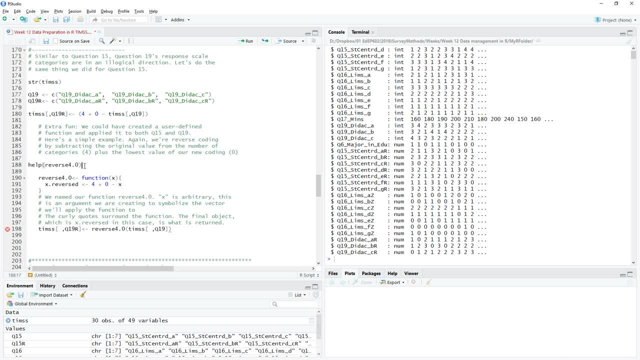 name you want to try out. I'm just pasting here and see if anything. anything shows up in R says no documentation for reverse 4.0 in specified patterns. Okay, I'm going to use the name that I just created. Let's see. 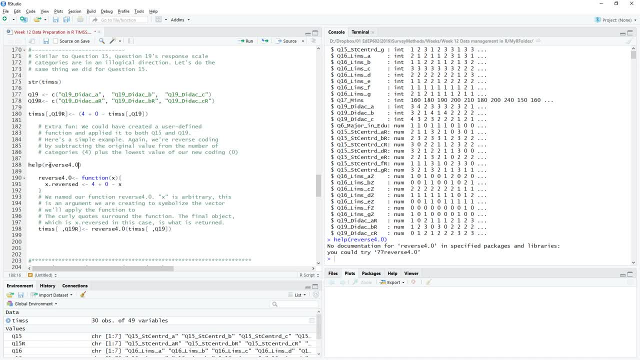 Okay, So I'm going to set it to to uh R. Let's see if that comes up. Okay, So you'll notice. oh, it's, it's. uh, it's a filter function. So I'm going to add a function where that's going to come up. 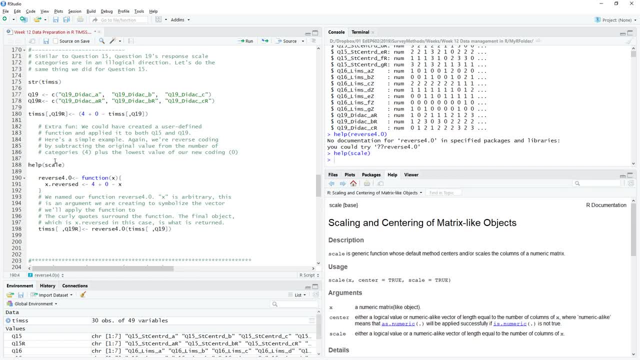 Okay, And what we're going to do is I'm going to use to have the R function for one of the operating instances and I'm going to set that to R. What we're going to do is I'm going to put this in here. 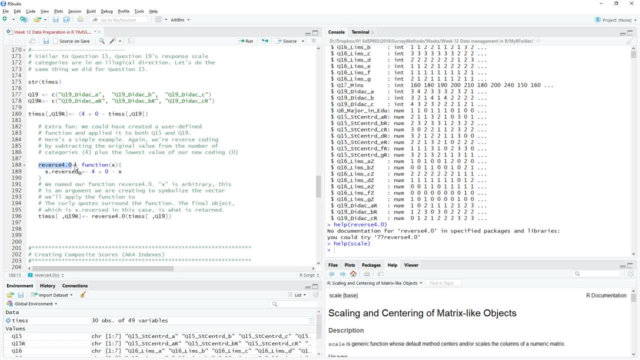 Right, Okay, decided what we want to name our new function. we actually create it by using, of all things, the function function And it sounds like a song. Okay, so here is we're going to have an argument, call it x, Let's have an argument. And so we could have a set of arguments if we 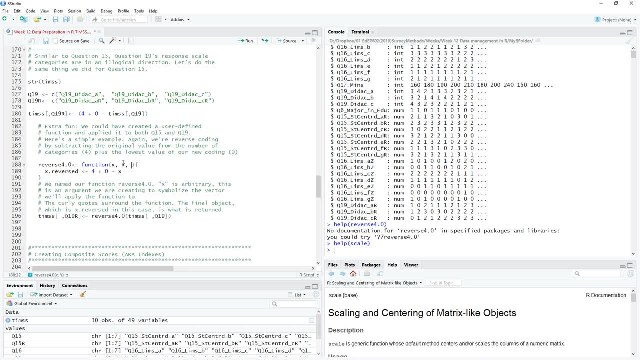 wanted. You know, we could have y, we could have data and so forth, But we only want to actually be concerned with one argument, and that is what it is we want to apply the function to, And so, within parentheses, after the function comes, our list of arguments. 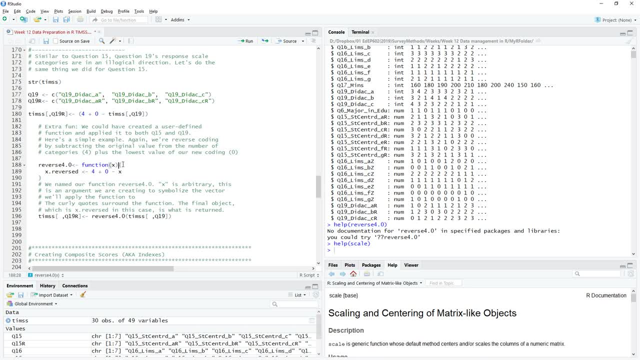 and separated by commas. Here there's just one. Following that, we have a curly bracket and this, traditionally, is displayed right after the function and at the very end of your function. R knows that it's done by that enclosed curly bracket. So and then? 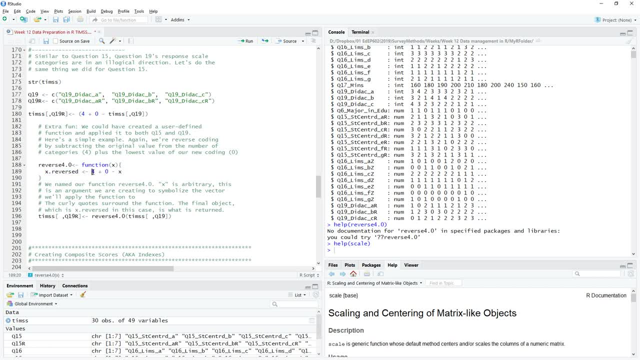 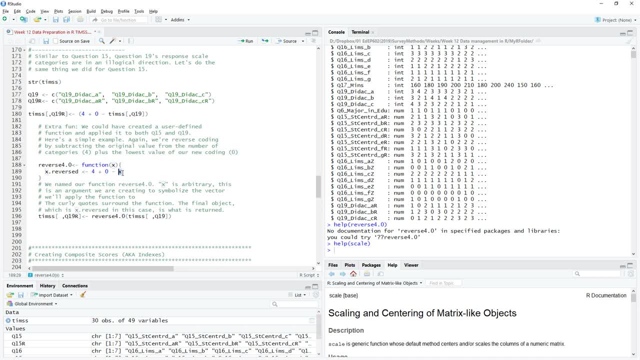 so it's the same minus x. Whatever x happens to be, we're going to assign something to x. So here, x was this and we're going to arbitrarily assign it to an object. I'm just calling it x dot reversed. You could call it my favorite output, I don't know. But 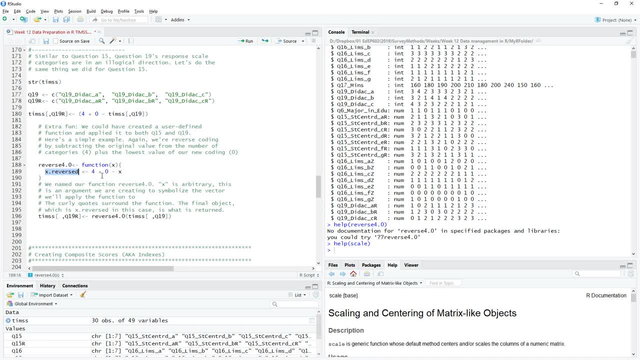 this final output is what will get produced by the function, and so if we use our function on x, here's x. we could actually do x equals if we wanted to be very specific, but we don't have to because it's the only argument, and then we apply it. 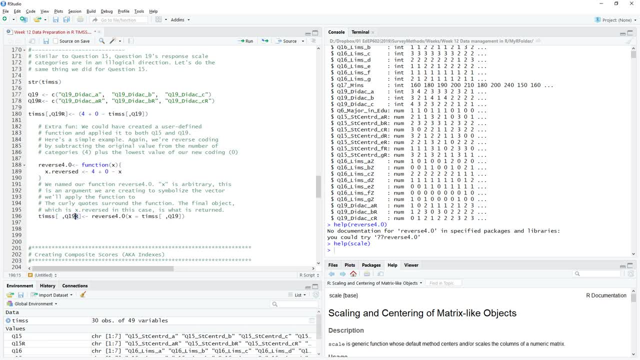 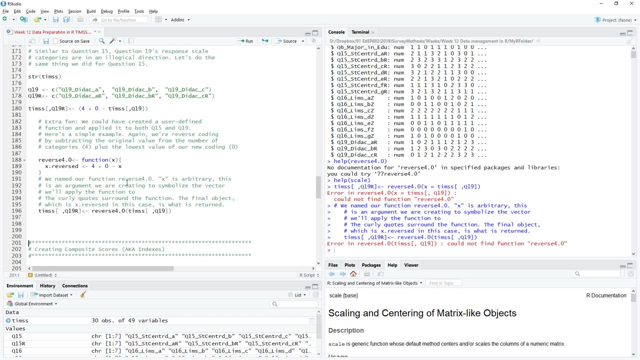 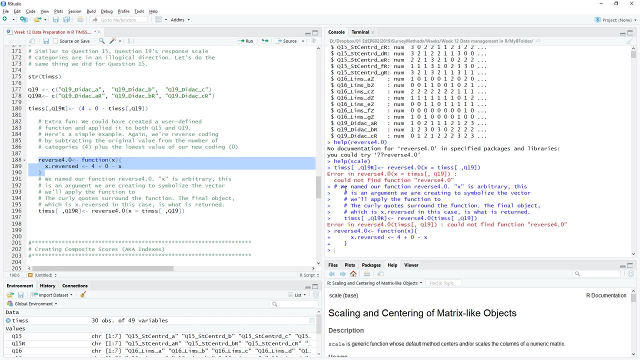 it then creates this new set of data. I could run this and it should give me the same. oh, it didn't work. Oh, it didn't work because I didn't actually run it. I need to run my function, Isn't that fun? So let's run it Now. r knows what reverse r means. 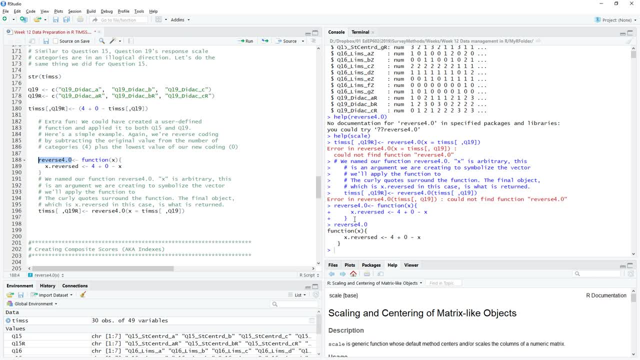 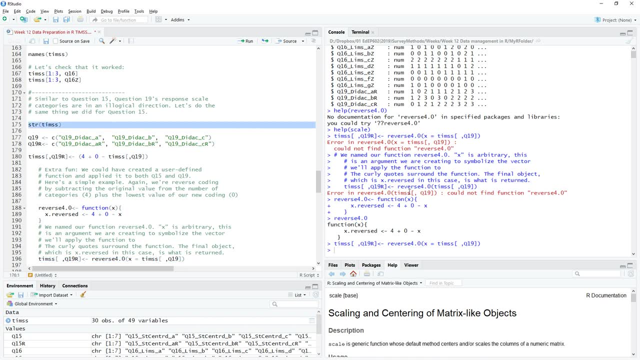 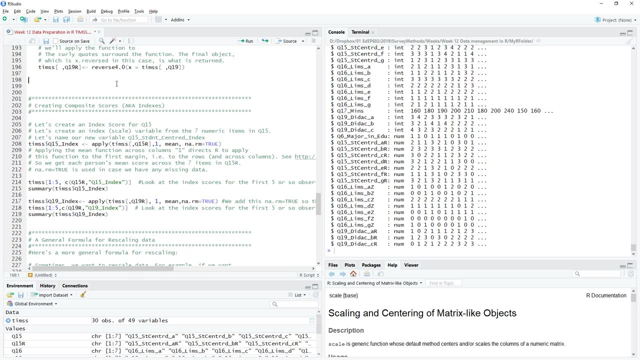 In fact, if I select that and run it, then it will show me what's inside of it. Now it should work. Okay, so I could go back to my structure function and find out that they are, as I would expect, like this. Next, let's create composite scores. 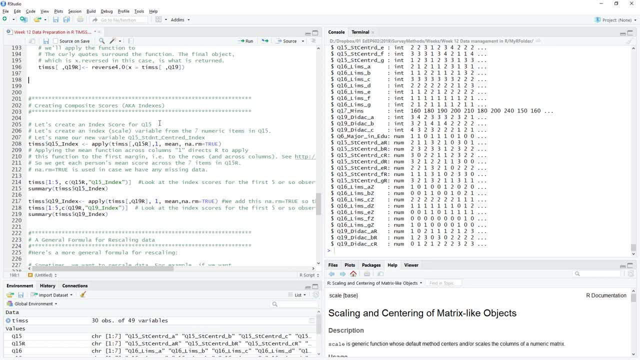 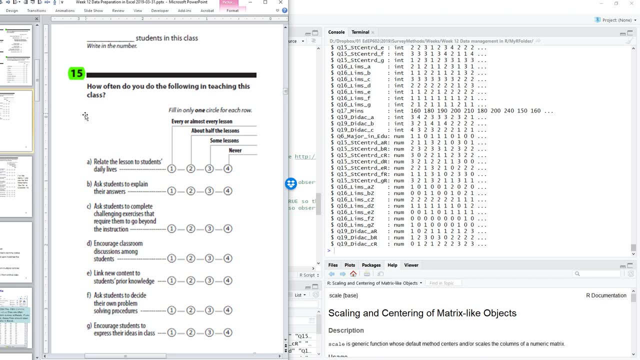 which are also called indexes, and so let's look at question 15,. and so this was about how often the teacher did this in class, and we had coded these from 0 to 3, 0,, 1,, 2,, 3, so I want to get each person's score across these. 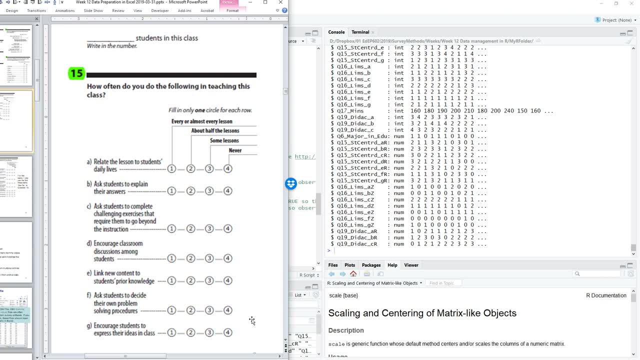 7, is that 7, 1,, 2,, 3,, 4,, 5,, 6,, 7, yeah, 7 sub-items. and then get a question: 15 composite score. that goes on a scale from 0 to 3.. 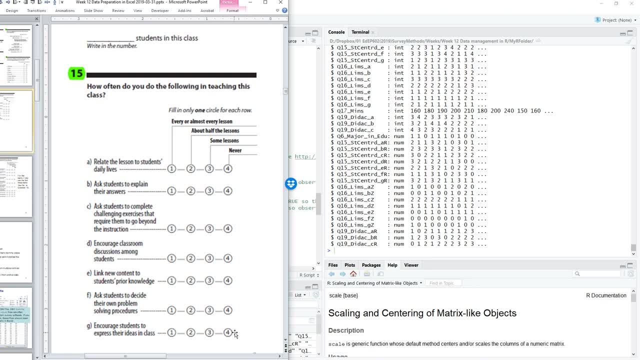 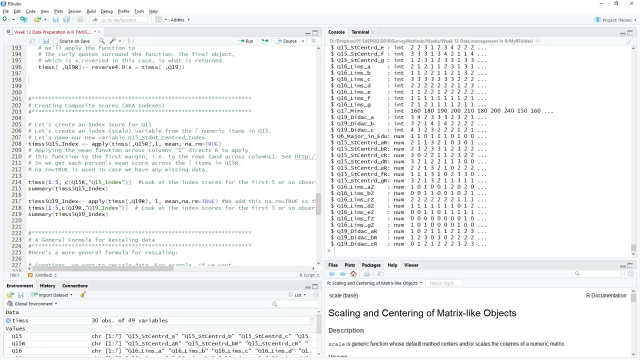 Some people, yeah, they add up the responses, but to me it makes sense if we keep it on the same scale. That way we can track their average response back to the meaning of the actual scale. So let's do that in r using the apply function. and this was actually explained. 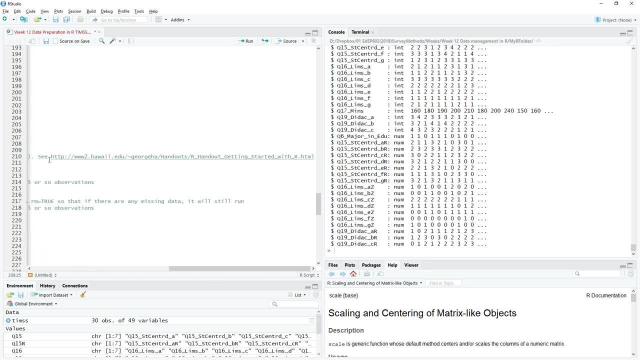 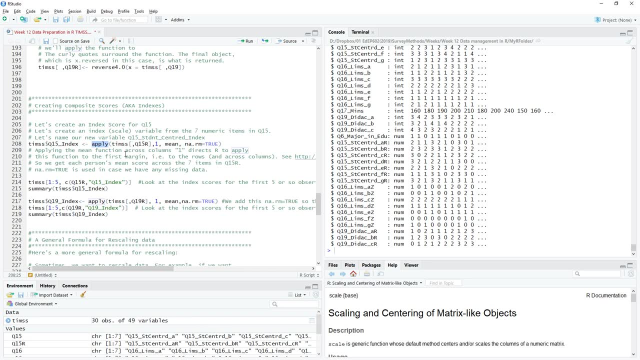 um in our lesson at the early part of our class and here's the link in the r code if you want to copy and paste that and and get um call that back up. But basically we're creating a new variable and I'm calling it Tim's Q15 index. 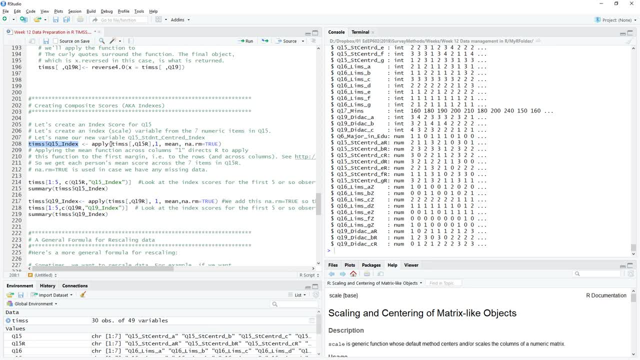 and to do this, uh, I am using those, those items or those um, um columns, uh, that were in Q15r. So remember, this is not in quotes because it's an r object, But if I, if I um, highlight that and then run, it'll show me what's inside of that r r object. 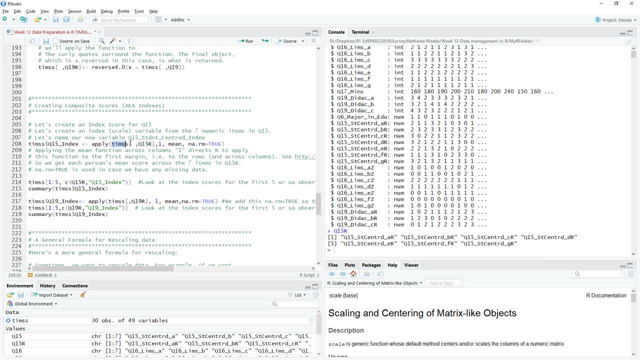 So, basically, what I'm saying is, with the Tim's data set for all rows and and for all columns that have these names, um, please perform the mean function across those columns And um, so this one is: stands. stands for the margin. 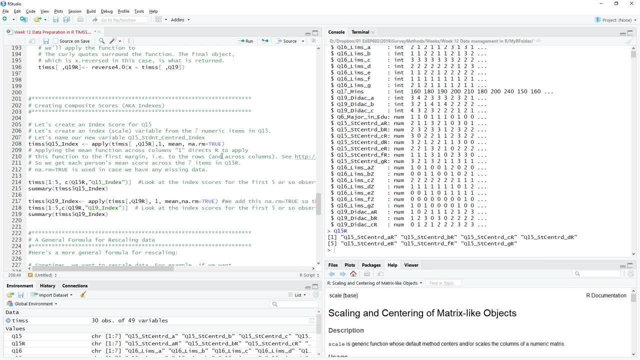 and it just means to apply this function to the rows, uh, rows being, I guess, the the first margin and columns being the second margin. So, um, we would perform the function across columns And this narm, that just means if it's missing. 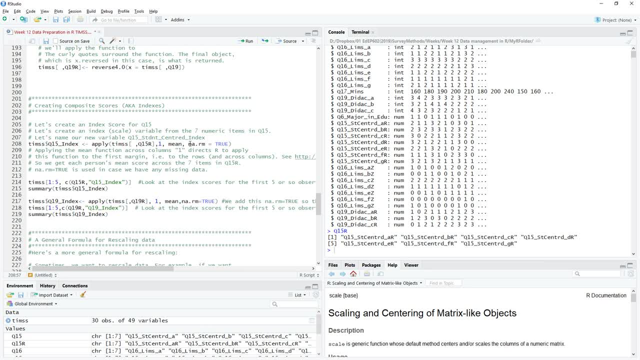 should we re, should we remove that um person from that calculation of the mean? Or rather, should we remove that not the person, remove the um, the item uh, from the mean? So if, if, if a person didn't answer number um, you know. 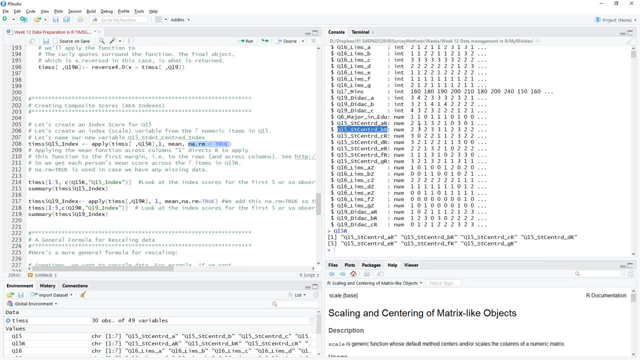 Q15br. you know, and maybe maybe person two didn't. so instead of a three- maybe it was na uh, then it would still calculate that person's mean across the other a through g items And therefore we get the score of that person. 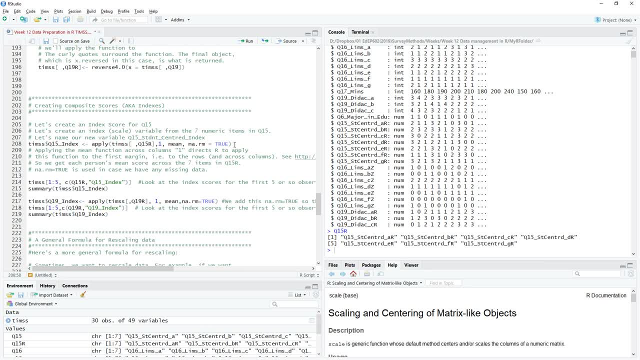 on those questions for which they answered, And it's still on the same scale of zero uh to three. So that's kind of useful if we have this. um narm, That just means if it's na meaning missing, remove it. uh, true. 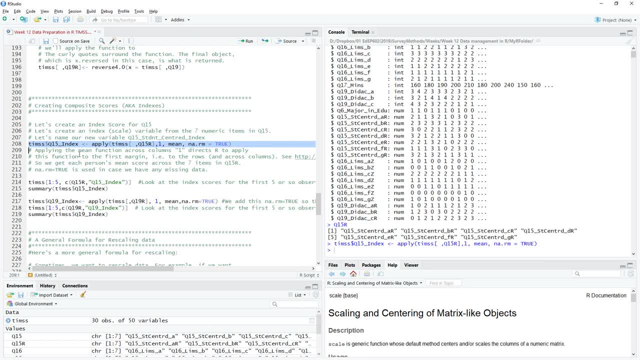 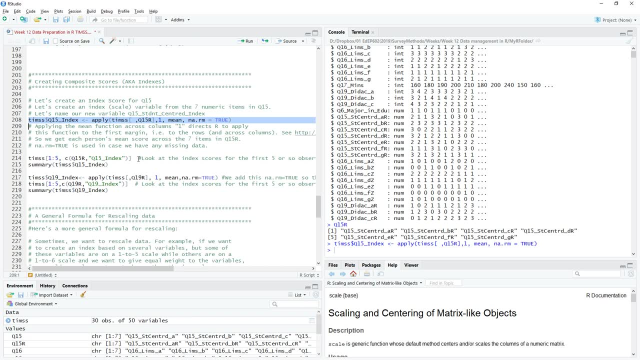 Um, so let's, let's run that, uh, and see what we get. So there's no error, That's, that's good. Um, let's see. So now I want to look at the first five. 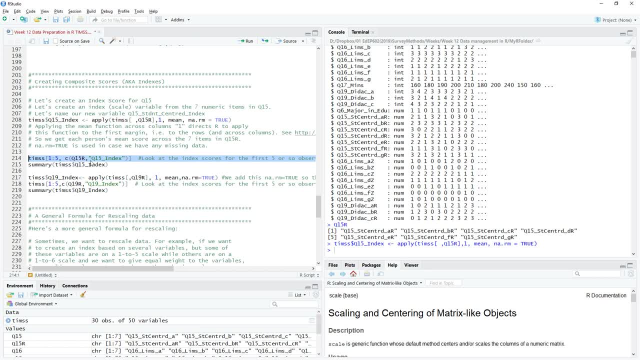 look at the first five rows of of data and look at the index we created, which is called Q15index. right here I like RStudio because if you highlight it, it shows you where that text is elsewhere in the text. 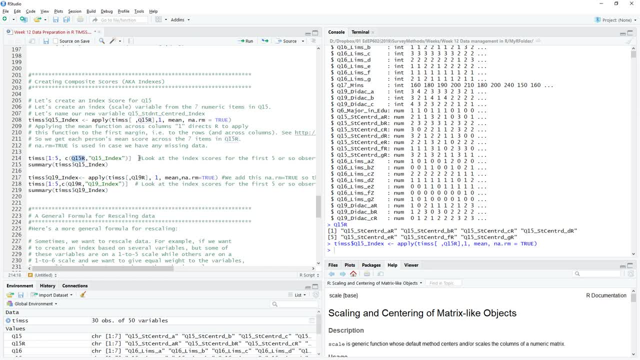 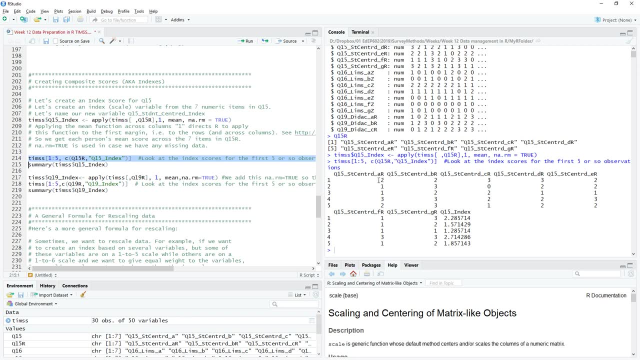 And I also want to look at the five questions that people responded to. So let let's do that. So for person one, they responded: two, two, three, or rather we recoded it: two, two, three, three, two, one, three. 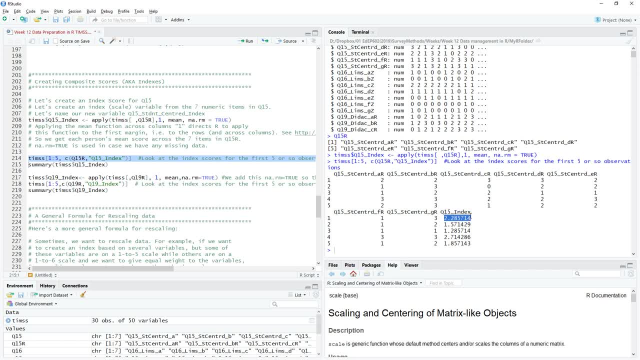 So if you add all of those up and divide it by seven, you will get 2.2857.. And that's the same as we have in our Excel file in the PDF demo. Um, and we can also do um. so so now we have a. 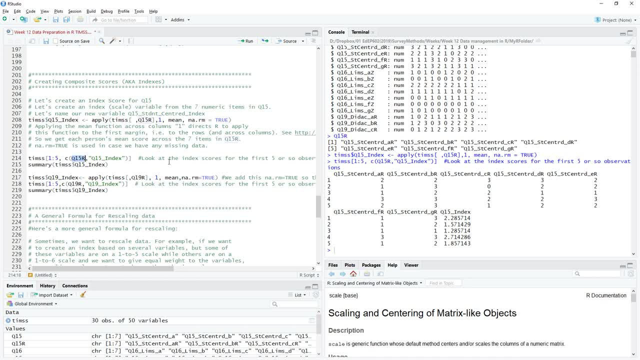 a variable that is more interval-like than our individual variables, which are more ordinal or categorical-like, And so it's it's easier or more defensible, rather, to perform statistics on interval-level scales, uh, when they are the dependent variables. 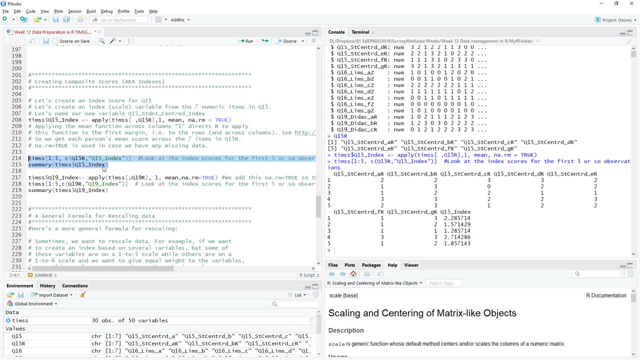 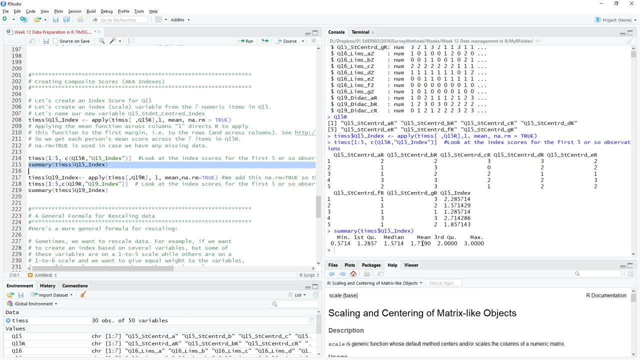 Uh, when they are predictors, we tend to get away with it by running a general linear model, But in any way, uh, let's. let's look at the um descriptive statistics And it looks like the average, the mean. 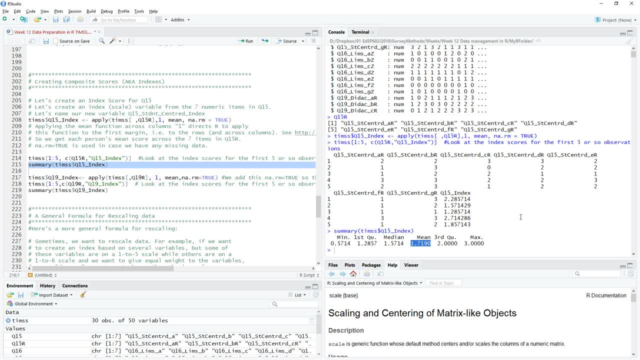 was 1.72 on that zero to three scale. Uh, uh, we can see, uh, we can see the average of how much uh teachers are using student-centered approaches in their classrooms, And we see the the min and the max. 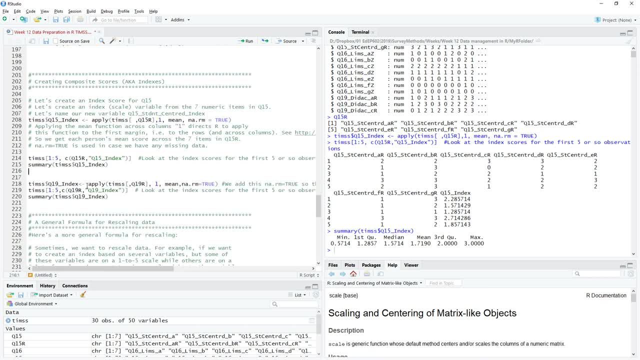 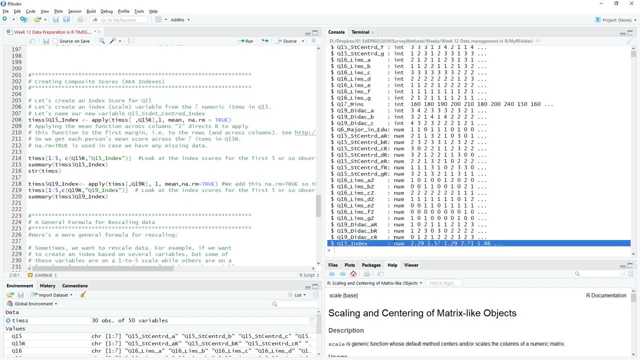 So we could also look at the structure of TIMSS again um to see what they look like. And we can see that our index is at the bottom because it's the last variable we created. It's numeric. We see, the first person's score is 2.29.. 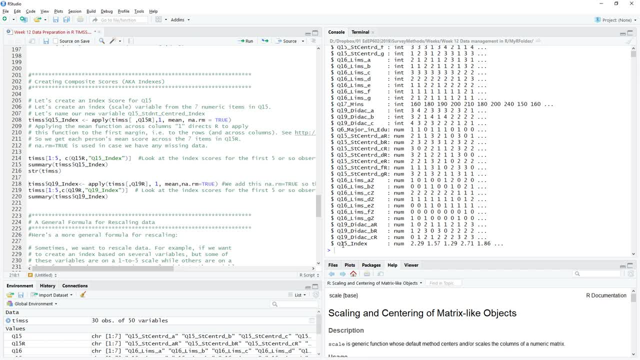 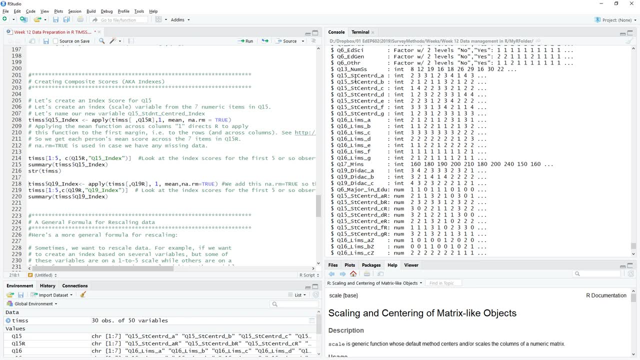 We see the second person's score is 2.57 on this composite index. So so this is what we can then use in our inferential statistics. So and again, you could scroll up and calculate uh for for this person: 2 plus 2 plus 1 plus 1 plus 2 plus 3 plus 1 divided by 7.. 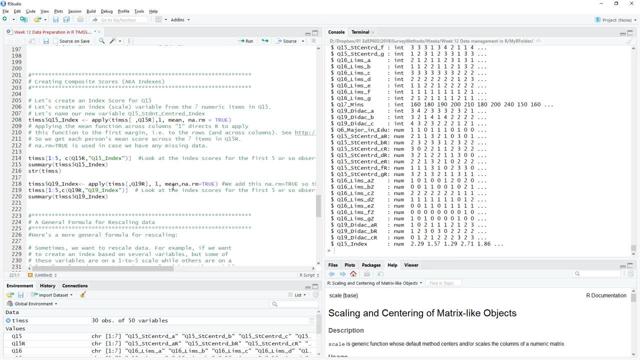 And that'll give you 2.29.. Uh, so that's a quick and dirty way to make composite scores. Uh, let's see, Let's do the same thing for question 19.. Uh, again, we're just using the same function. 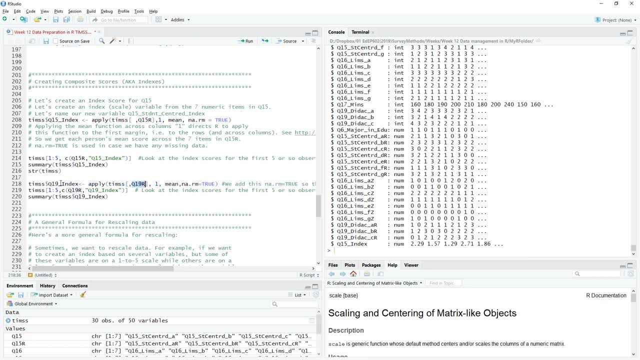 Just, I just replaced Q15R with Q19R And I changed the name from Q15index to Q19index And I can perform all of those same functions and see what the mean is there, which is a little bit lower. 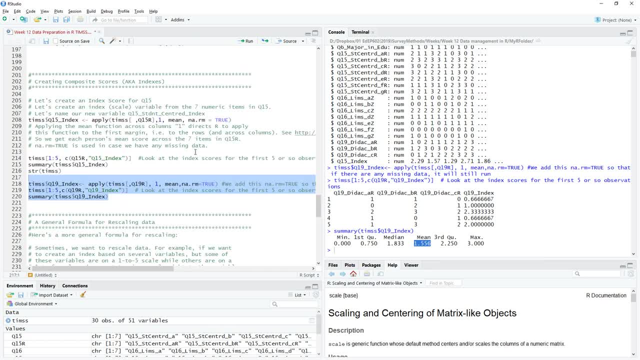 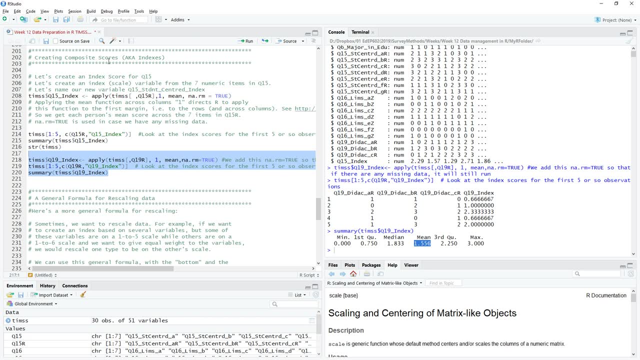 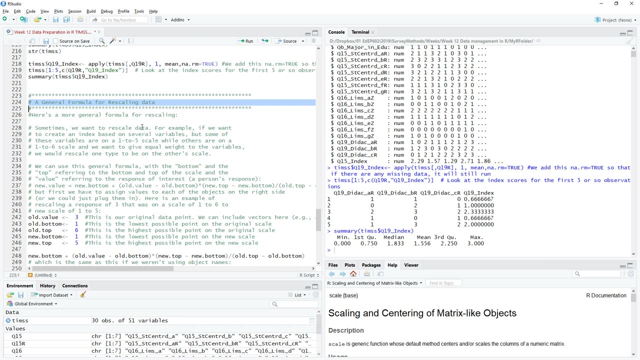 So that, I guess, covers those three main points. um, which was managing data in R, Rescaling the responses and then creating composite scores. Um, here is a general formula for rescaling data, And this is in addition to- it's like an extra to what is in the Excel file. 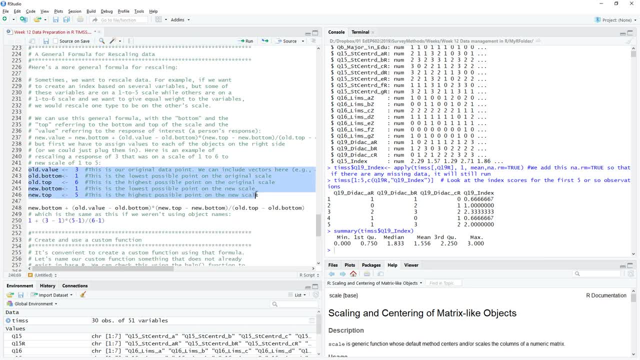 But I I provide this general equation for um transforming your data from one scale. So if it's, for example, if your old scale is on a 1 to 6, uh scale like the Likert type scales. 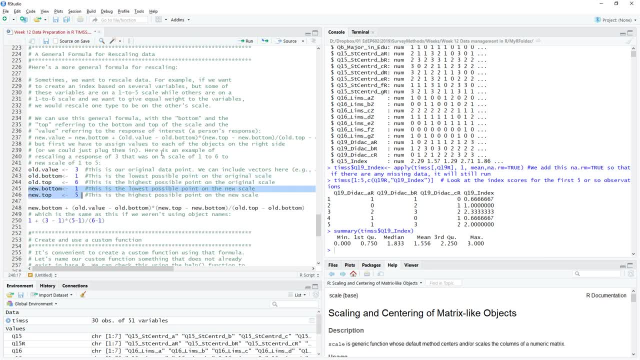 and you want to change it to a 1 to 5 scale. you know, if you want to actually um, combine two, two, two types of items that are on different scales and put force them to be on the same one, 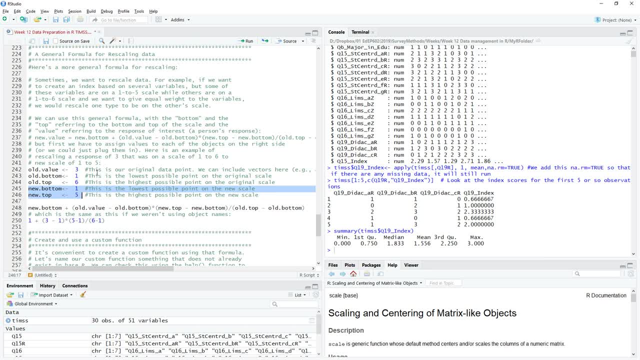 and then create an interval level, um, yeah, variable from those, then you would want them to be on the same scale, So so this helps if you turn some of them into the other one's scale, And so here's the general equation. 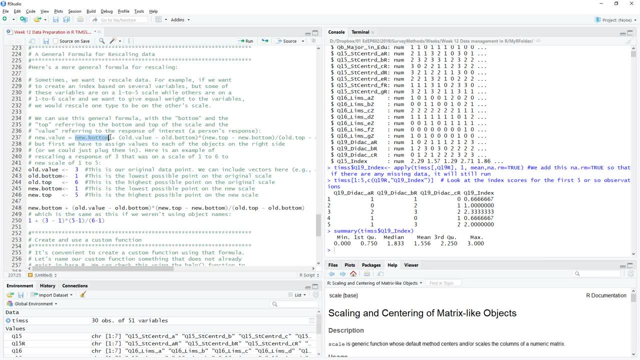 Basically, your new value Will be the new bottom, The new bottom being- uh what? the bottom? the lower end of the scale you want to be in your new, you know um- system. So like zero is what I like as a new bottom. 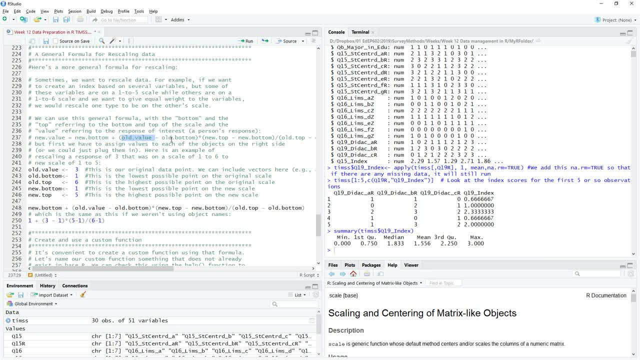 Your old value. that's the actual score or or response that somebody provided, minus the old bottom. Multiply that difference by the new top minus the new bottom And divide all of that by the old top, By the old top minus the old bottom. 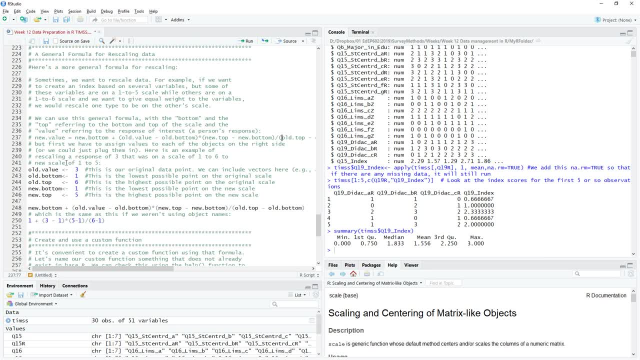 So this function, uh, we can use after we have assigned values to it. So say, I'm going from a one to six scale, A person got a three And I want to put that person's answer of three on that one to six scale. 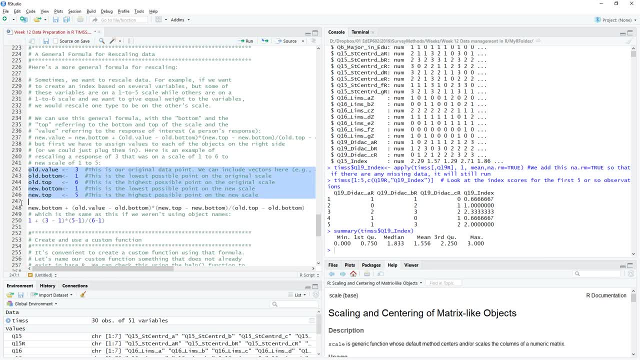 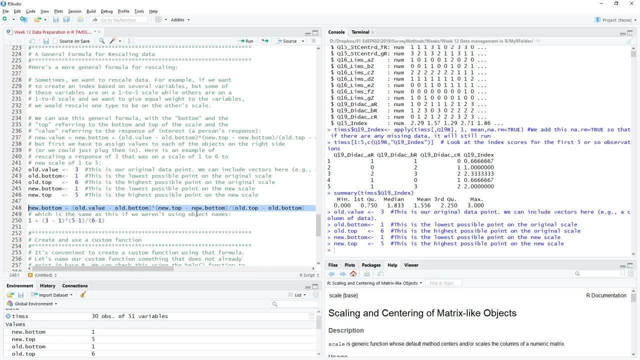 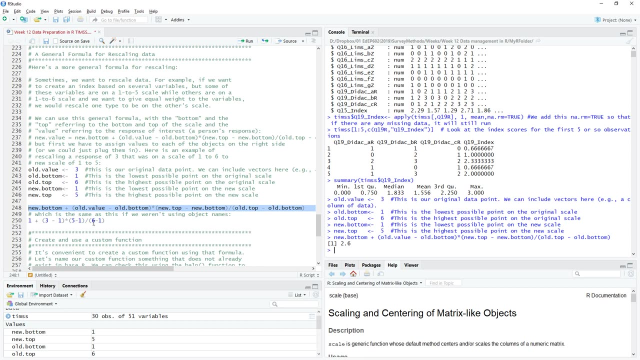 on the scale that goes from one to five. So, um, you can replace any values here And perform this function here And you'll get the result, which is 2.6.. So it is lower because the one to six scale is broader than the one to five scale. 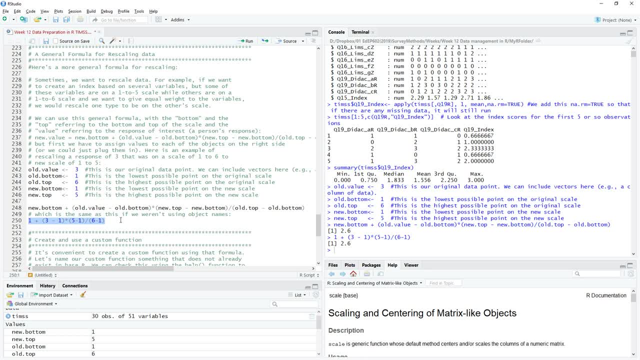 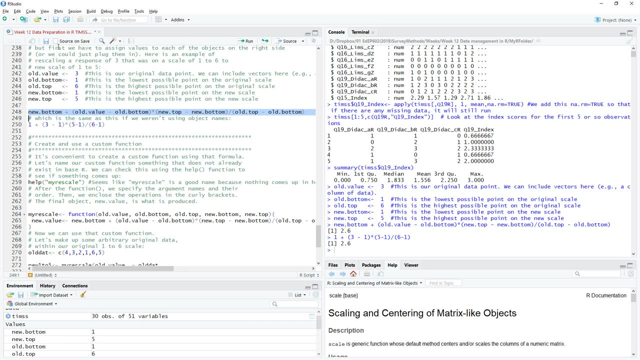 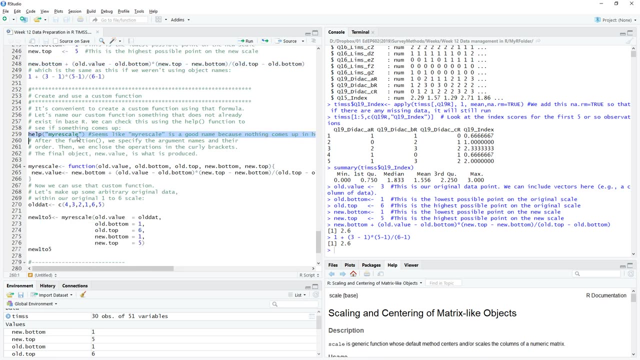 And I actually hand calculated it and get the same response here. So this is valuable for um lots of different purposes in survey research. Uh, let's see, I can create my own user made function from this. Maybe I'll call it rescale. 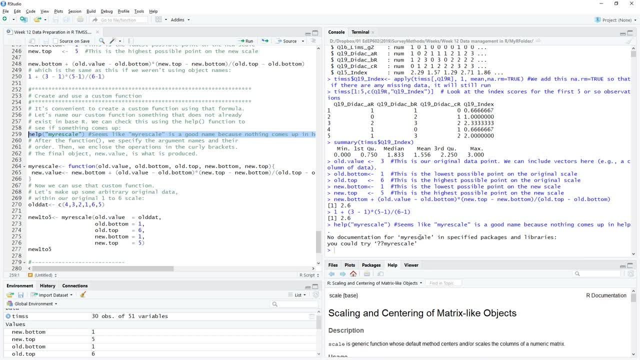 So I'm going to do a help and see if there's anything called rescale. No, that means I can use it, And so now I have a whole bunch of arguments in my function. I've got old value, old bottom, old top, new bottom, new top. 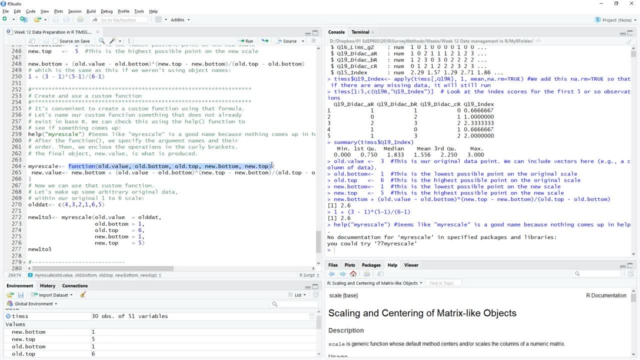 And those are things I have to specify when I perform the function on some data And from my function the new output will be the new value, And I can perform this function on uh, a vector of data, Like you know, an entire um column of data. 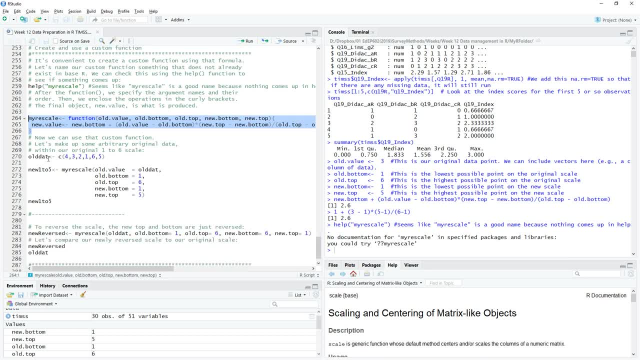 And create new um, new variables. So let's say I have these old data And they are on the one to six scale. So let's say the first person got a four, The second person got a three, The third person got a two, and so forth. 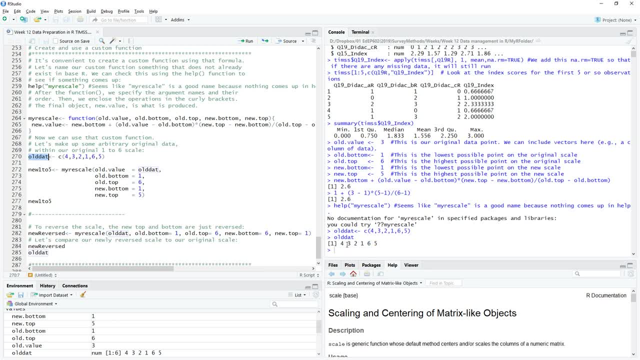 And so I can click on my old data after I have run it and see that it's there. I perform my user made function on that, But I have to specify what my values are. That's the old value. This would be like what x is in the other function. 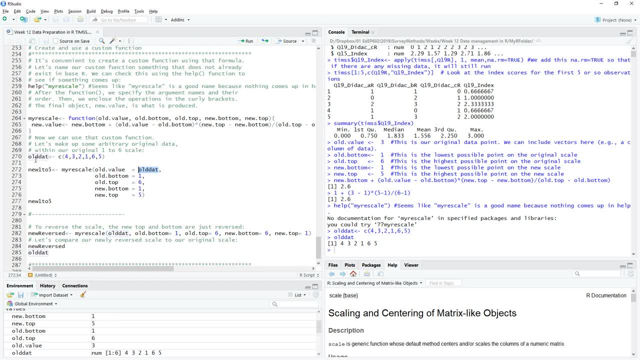 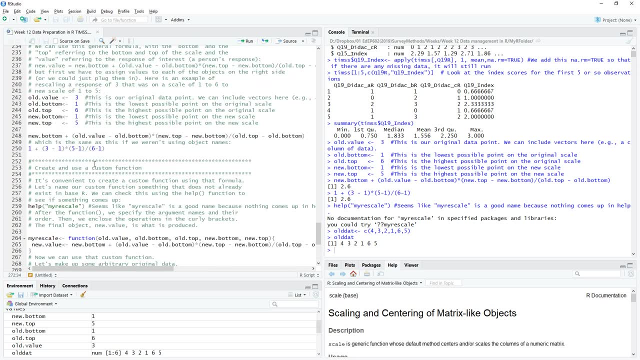 Or the old data. So the old data is this object here. So now I have a vector. Uh, you could have a column of data. So it could be something like um Tim's. you know, if you had a variable there that was like Tim's um 22.. 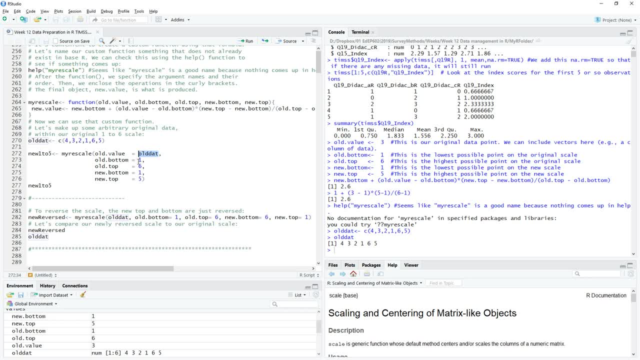 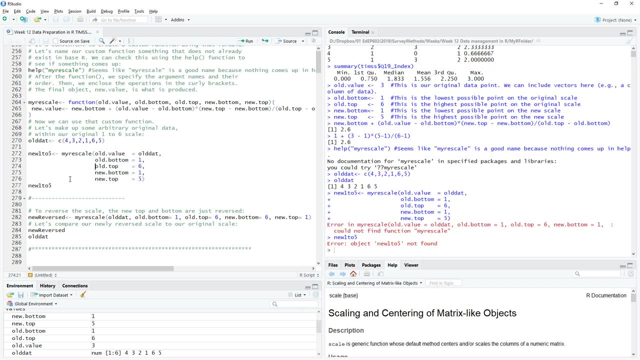 You know, it would be like the 22nd variable or something like that Um and uh. so I'm specifying the arguments And I should be able to perform that calculation. Let's see. Did I do everything correctly here? 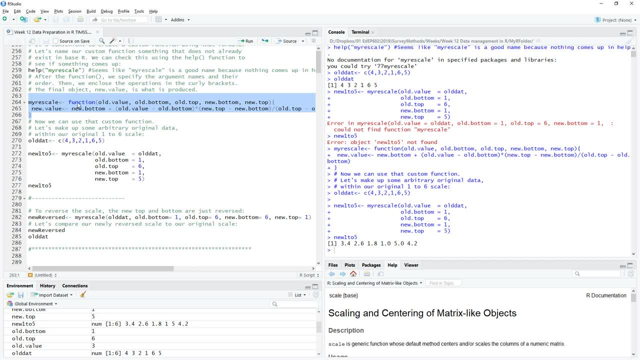 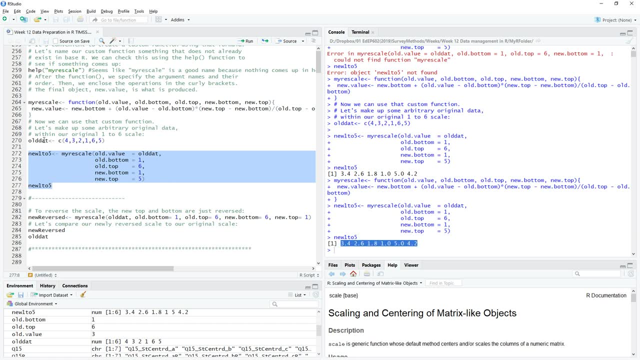 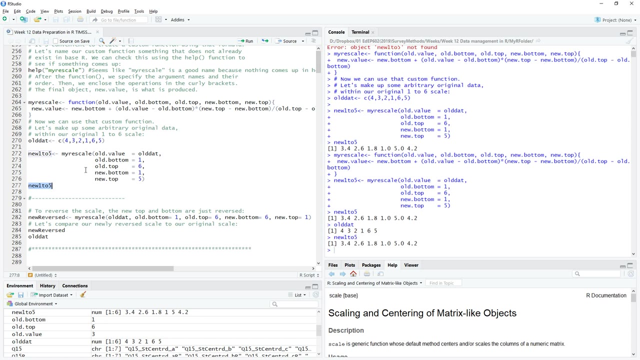 Yeah, I guess I didn't um run my. I have to run the function right before I then call it up. So running the function will then give me my original data rescaled to my new data, And if you hand calculated that these are the responses you would get. 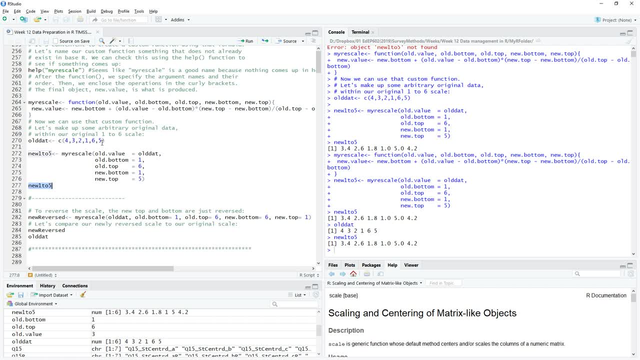 So this is really valuable when you have a large set of data. Uh, and it also demonstrates how you can create your own functions. Um, So I can use this, So I can use this function that I have created to also reverse the scale. 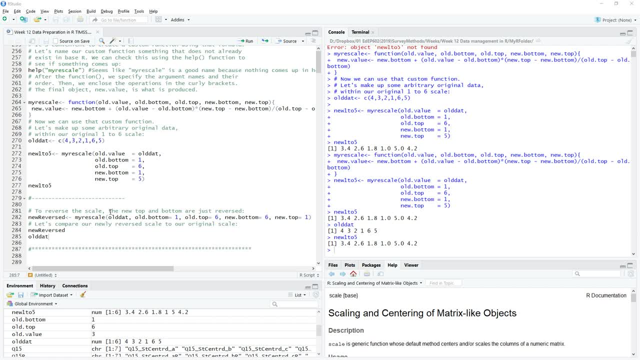 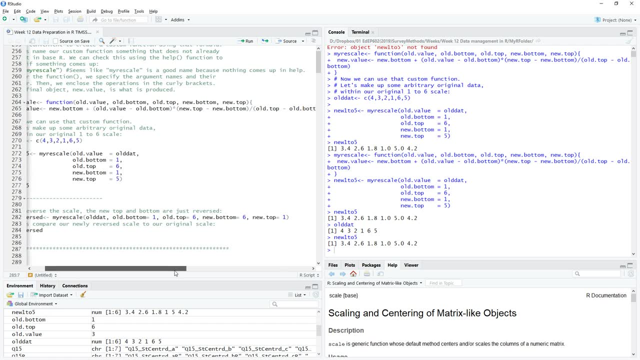 Um, it's a little bit overkill for just reversing a scale, But basically, um, we want to make sure that the new top and the bottom are just reverse of each other. So you can see that the maybe my in my old data maybe the old bottom is a 1 and the new yeah, and the old top is a 6.. 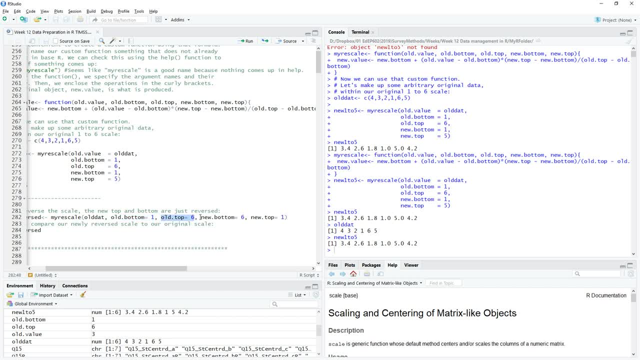 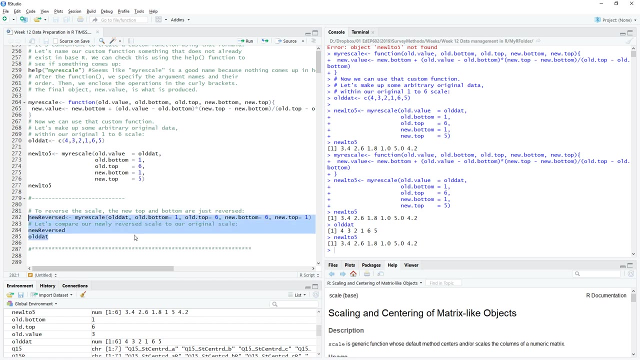 And I want to reverse it so that the old, the new bottom is a 6 and the new top is a 1.. So this just reverses it. Yeah, so the bottom becomes the top and the top becomes the bottom. Um, and that will give you. I guess we can compare those. 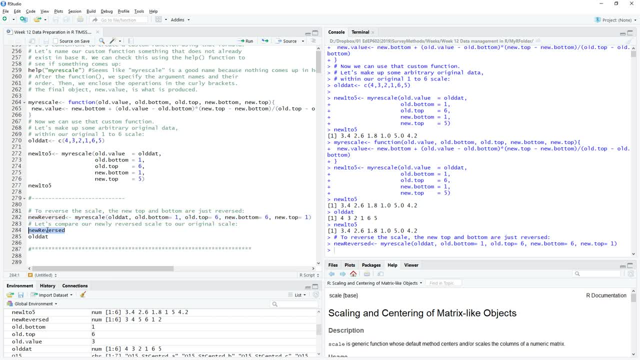 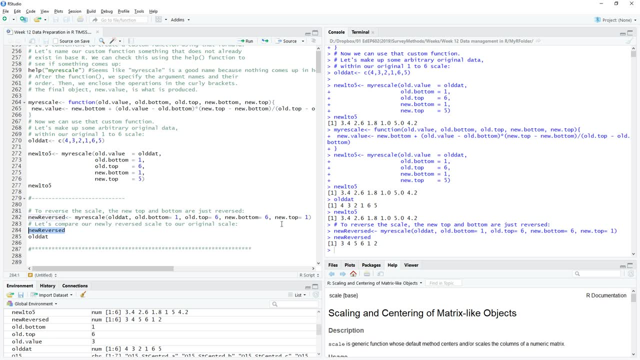 So let me, let me run that, that line, And then I can call up that new object that I created, which is, you know, the vector values. So on the new scores. so person 1 now has a 3, person 2 has a 4.. 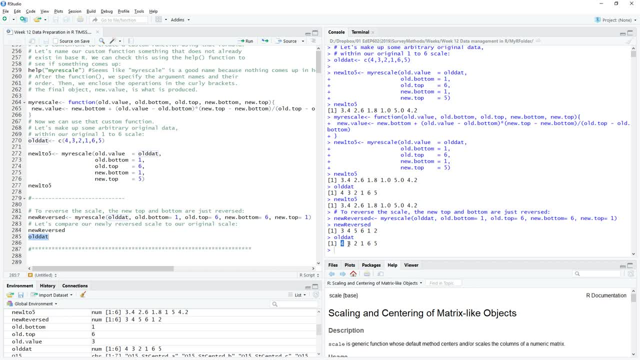 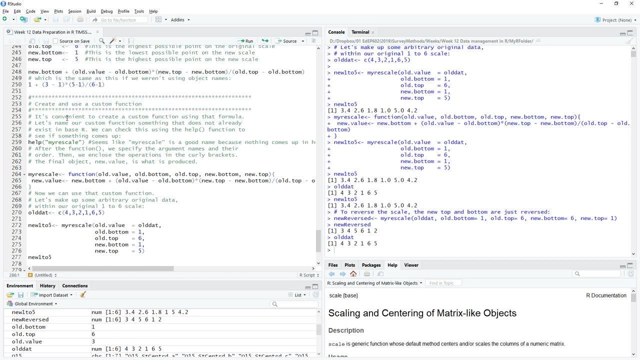 And here are my old data: Person 1 had a 4 and person 2 had a 3 originally. So you know, if you don't want to use that function above, uh, with questions 15 and 19,. this is another way to to do. that is just to have a general rescaling function.